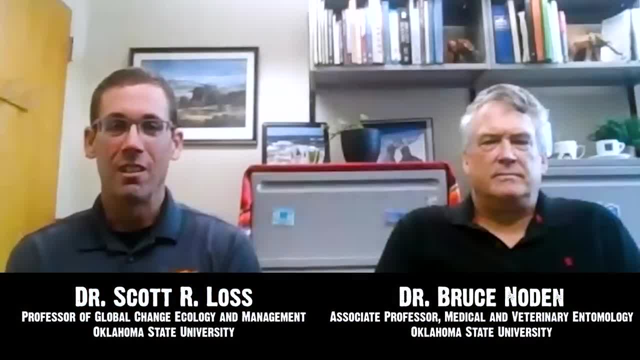 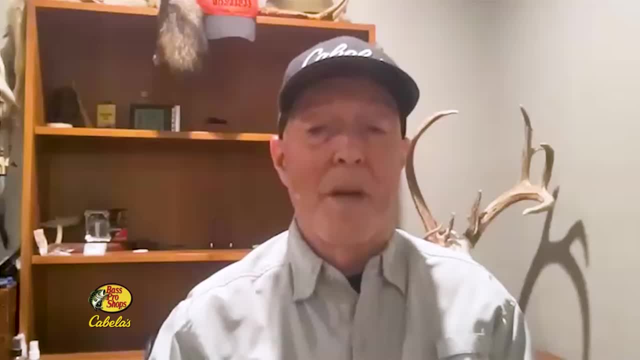 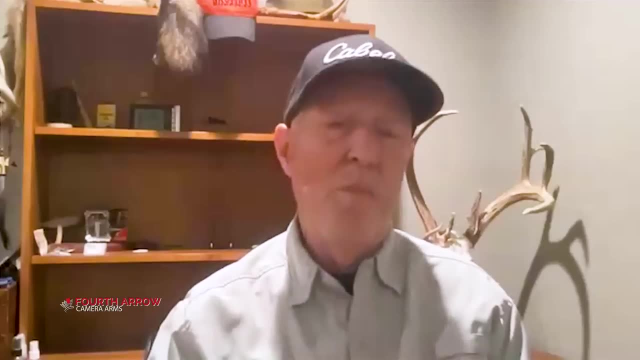 potentially contributing to carrying birds, contributing to carrying ticks, including in relation to this issue of eastern red cedar encroachment in the grasslands. Yeah guys, that's a big issue. So I've shared before but it's not widely known, but the numbers 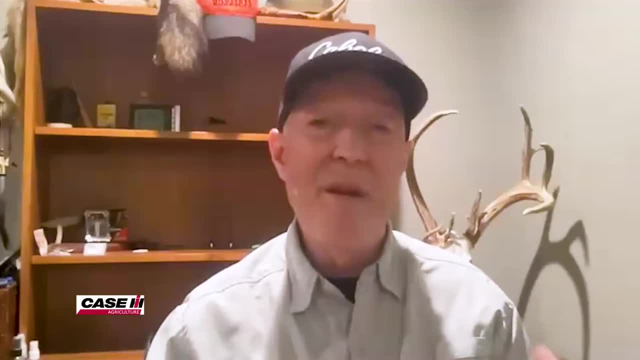 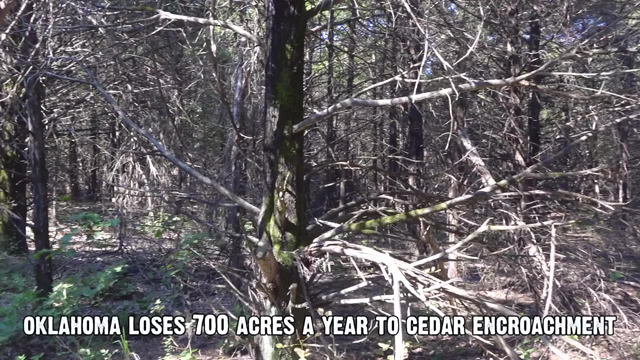 that the state of Oklahoma puts out is that they lose about 700 acres a year to cedar encroachment. and that's When I say that in seminars. some people- I can't you know- I think they think of one 700-acre block. but if you take the state of Oklahoma and cedar seed being dispersed, 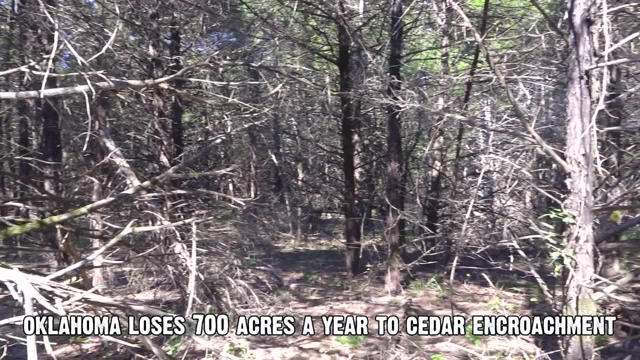 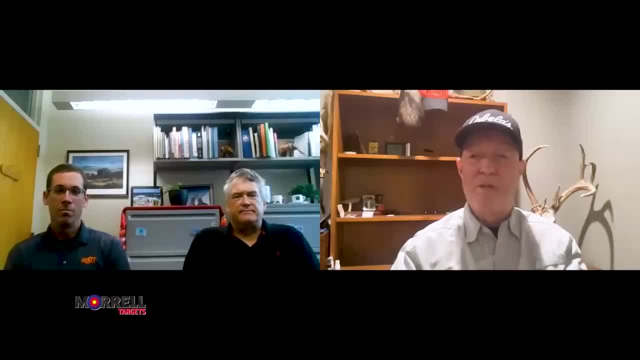 here and there and yonder. it's pretty easy to understand, without good treatment, Of course. prescribed fire or wildfire back in the day is what kept cedar at bay and when we've excluded that cedars are really spreading. Is that true? 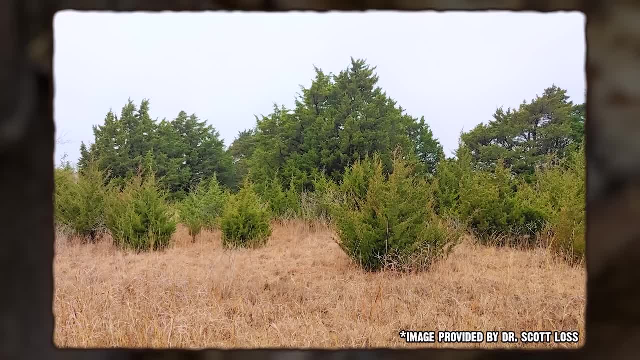 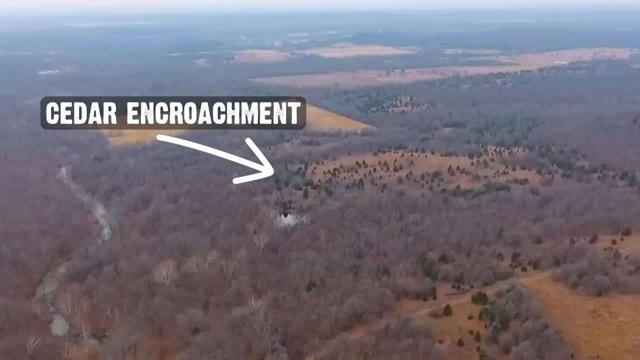 Yeah, certainly A lot of our prairies and shrublands and even more open oak woodlands are being encroached upon by eastern red cedar, especially in this region. It's an issue also like going on Great Plains-wide and even worldwide in open grasslands and savannas. 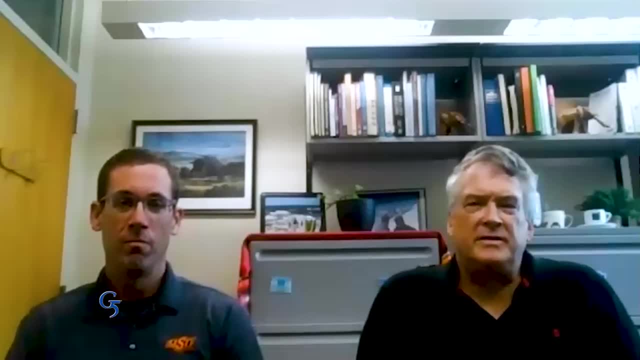 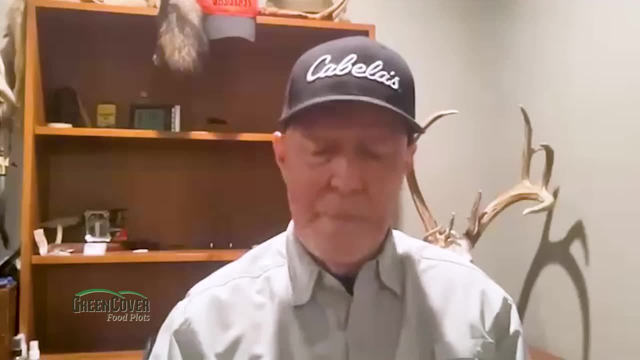 this issue of woody plant encroachment. Well, all it takes is a trip up I-44 there in Missouri and you've got the issue as well. Oh, we do, we do, And unfortunately, a lot of people here just believe cedars are always here. 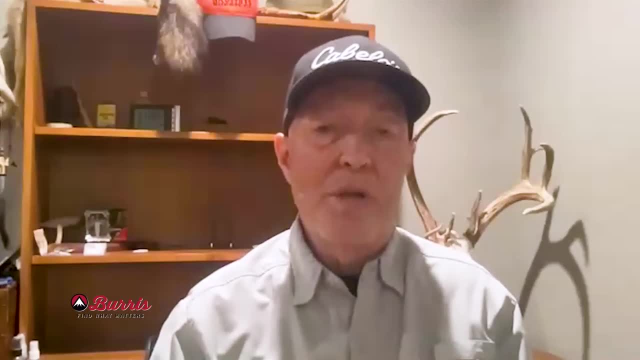 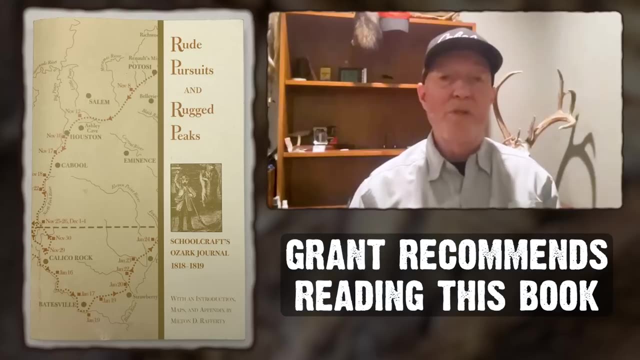 and I point them back to some of the early explorers that went through here. almost like Lewis and Clark, but smaller scale, obviously. One guy that went right through my area was looking for sources of cedar And he kept a journal, like Lewis and Clark, and a couple things he never mentions in the journal. 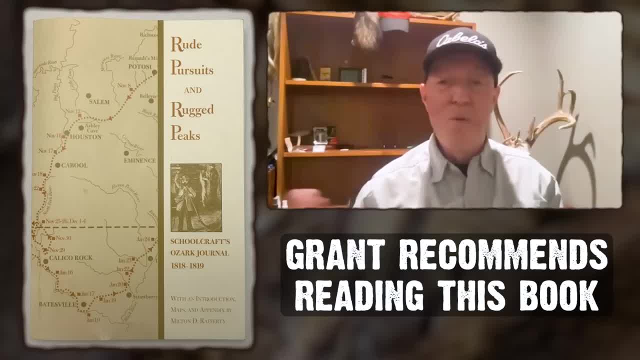 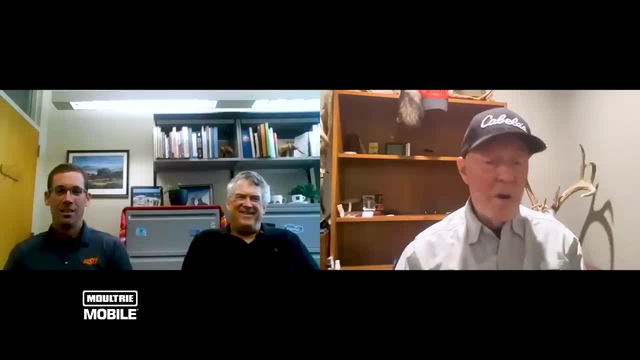 which I find fascinating is ticks One. if you walked through, you know 100 miles of the Ozarks now. you would talk about ticks Unequivocally. you would talk about ticks. And Lewis and Clark, of course, don't mention ticks. Most of these explorers never mention. 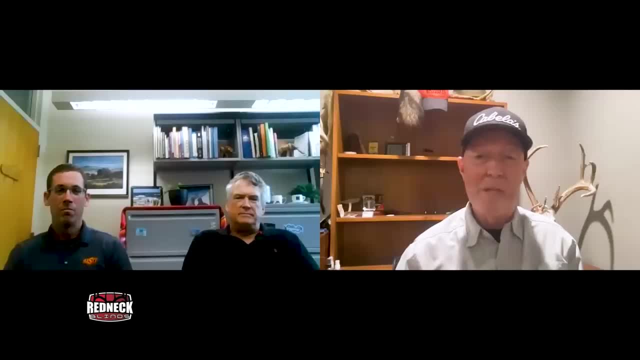 ticks, and they don't mention the preponderance of cedars. They talk about species and all the native grass and the woodlands and the savanna habitat. They don't talk about cedars. So we've lost that component of our habitat which let more sun in didn't make as friendly of an. 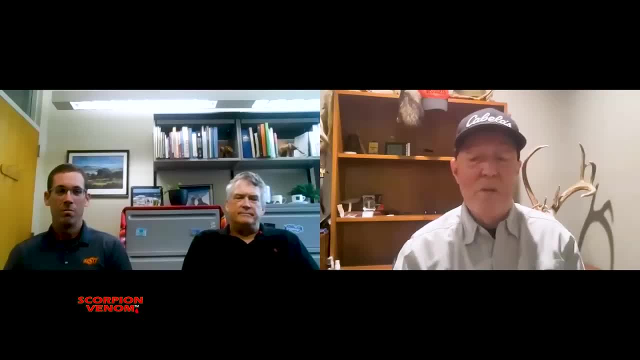 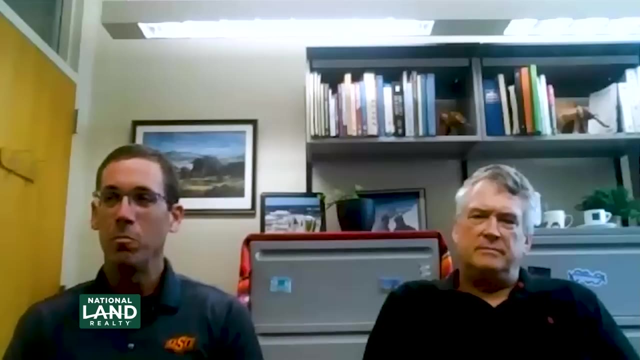 environment for ticks, as cedars do. So share with you know what you see in Oklahoma and how this cedar encroachment is actually causing a lot of ecological changes When a open grassland or a shrubland or an oak woodland like a savanna-type woodland, 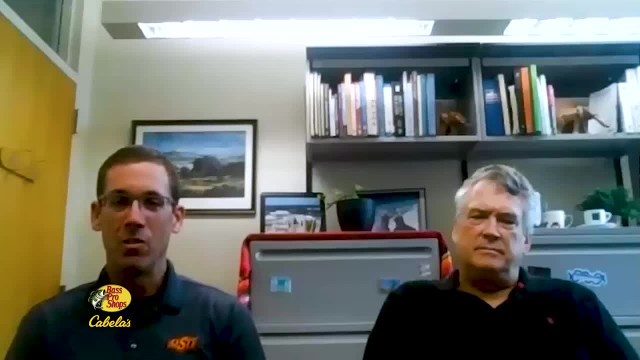 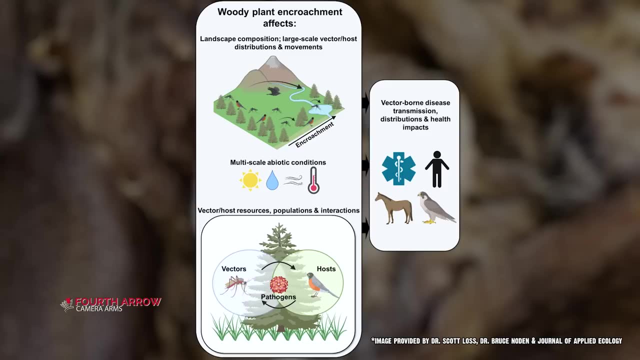 experiences eastern red cedar encroachment. there's a wide range of changes that happen from just cedar to cedar, So we've lost that component of our habitat which let more sun in just the condition, the abiotic or weather-type conditions, like the moisture, the air moisture. 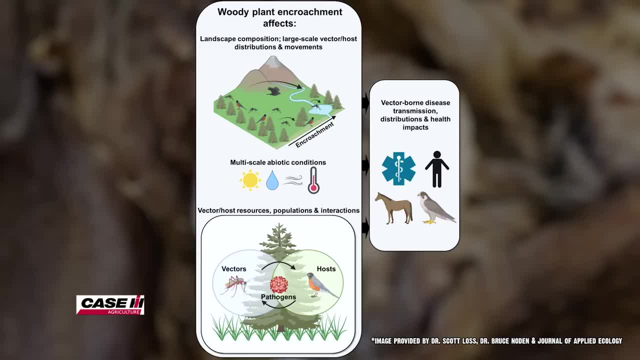 the relative humidity of the soil and the air makes it more humid year-round on average. under these trees can change the wind conditions, can change the temperature, solar radiation, all things which influence vectors like ticks, like Dr Nodin's studies, as well as. 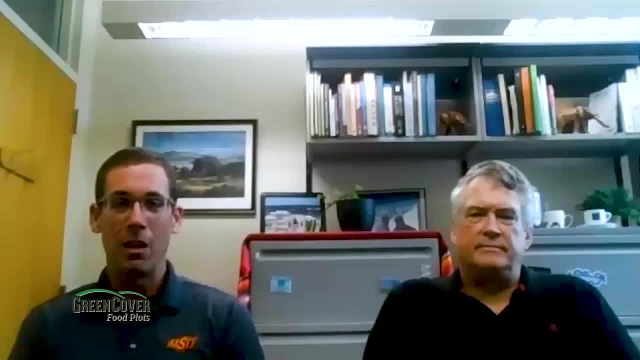 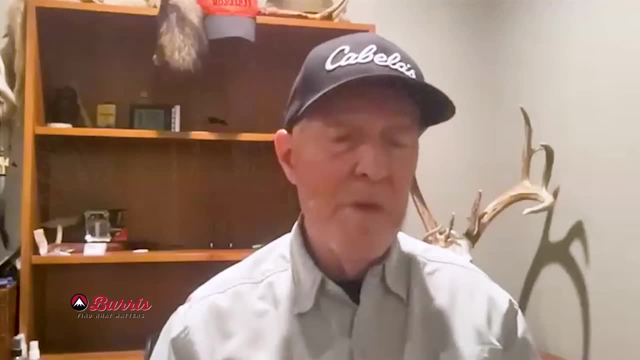 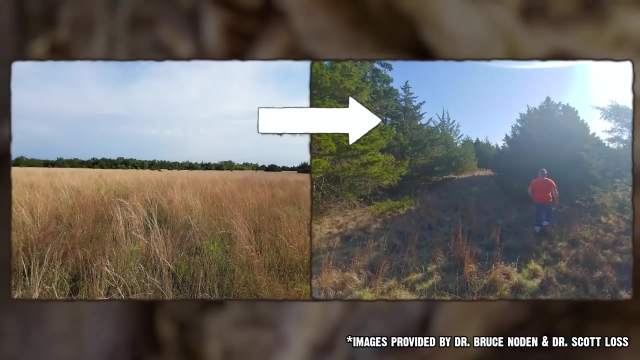 wildlife right will change the way different species of wildlife use the landscape as well. Yes, exactly, And that shading factor changes the plant communities drastically. So for the deer hunters like myself included, we're going from a forb and grass habitat to a shaded out habitat. 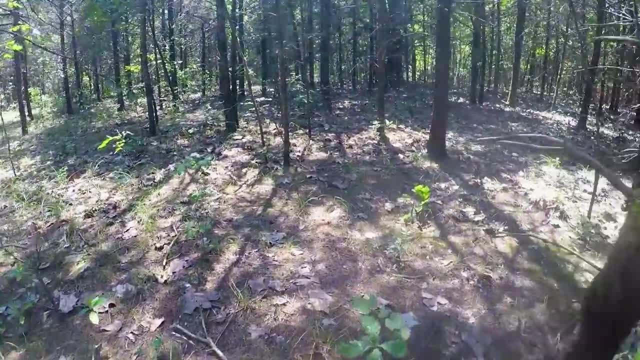 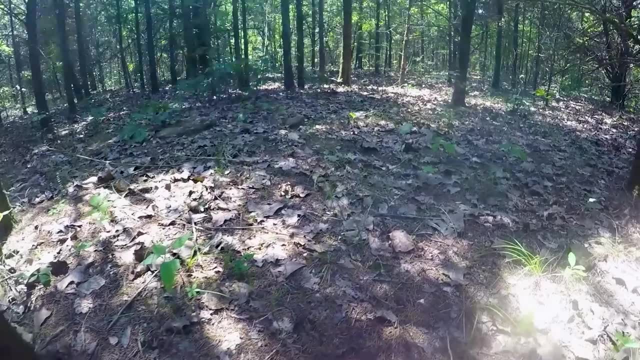 which is a significant reduction in habitat quality And antler size, by the way, because we're just reducing the amount of groceries, but that higher moisture content and shade is very favorable for ticks, So we're going to have to change that. So we're going to have to change. 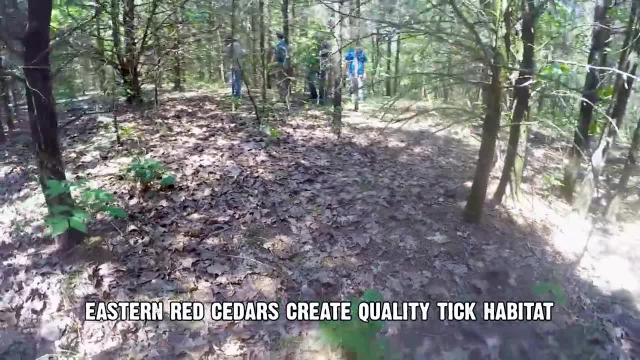 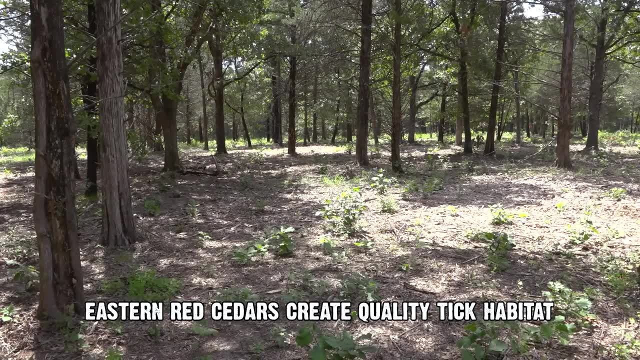 that And I like to share that, we manage populations of wildlife by managing the habitat, not the critter necessarily, And we're making very favorable habitat by allowing this to happen For ticks. we're expanding those populations by allowing this habitat to change. 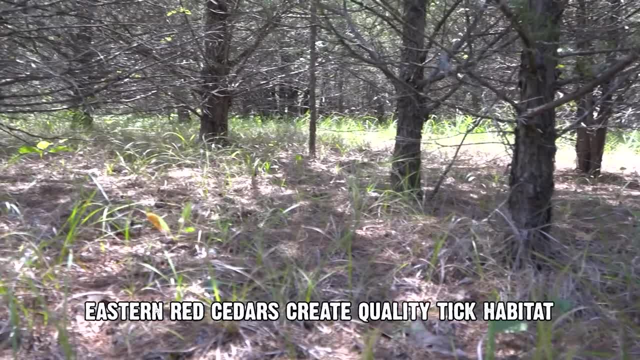 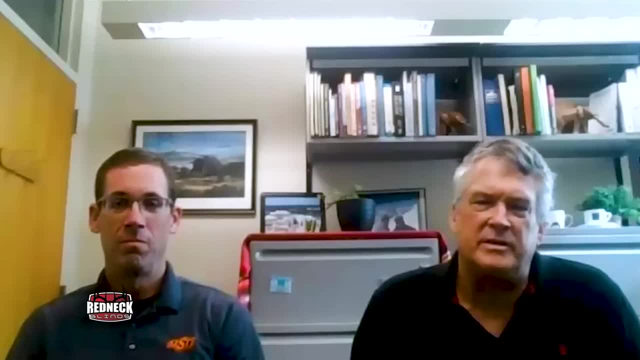 from a hostile environment to ticks to one more favorable. Do you all agree with that? You're correct about the open spaces. You know the sun comes in, the air starts moving, it dries out, the leaf litter, And you know. 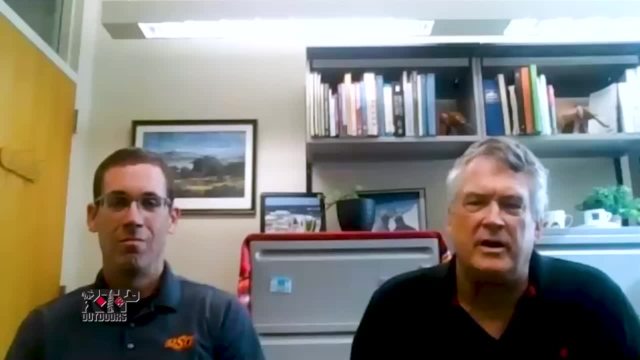 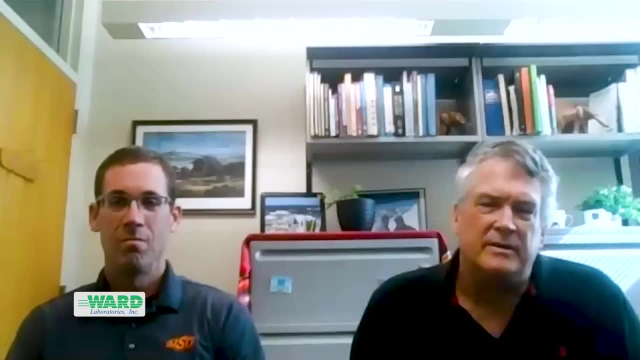 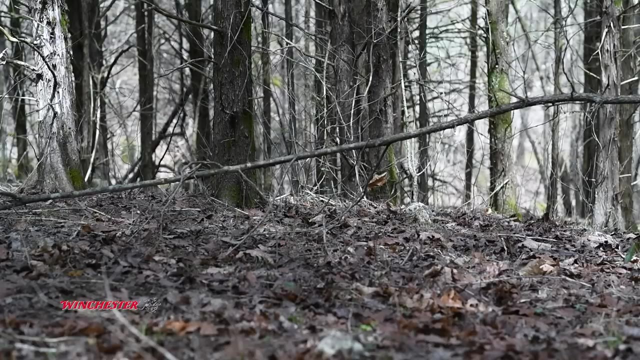 there's nothing that a tick fears more than dry air, And you know, if we can create spaces where the air is dry, then ticks, they're going to die because they can't handle the low humidity, And so what these plants are doing is it just creates these zones of higher humidity across the 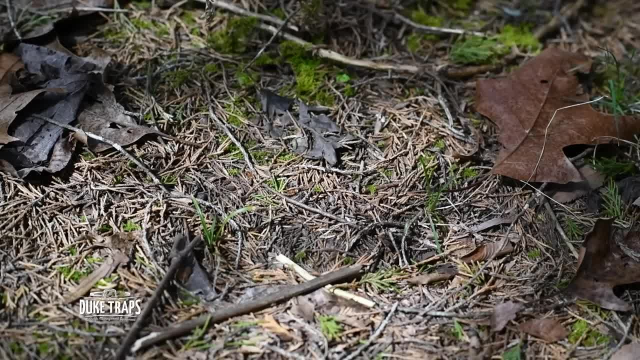 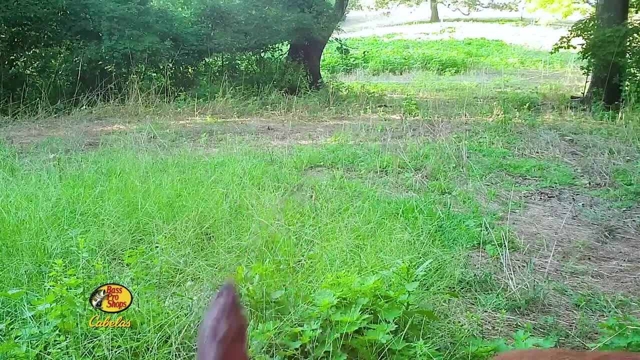 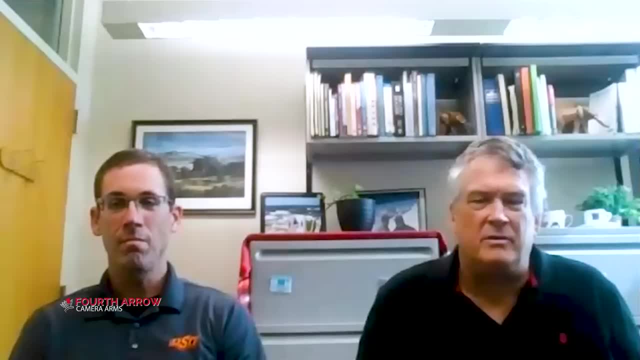 The question is, when they do, when they fall off of a deer, are they going to fall into a habitat where they can actually survive and lay their eggs and live? And normally, and particularly in western Oklahoma where it's dry, we've said no. You know, it's been dry, The ticks fall off the 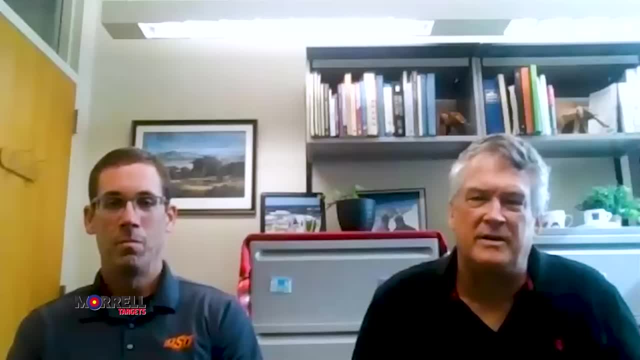 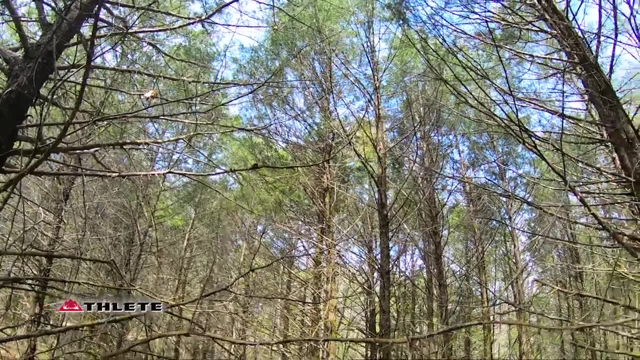 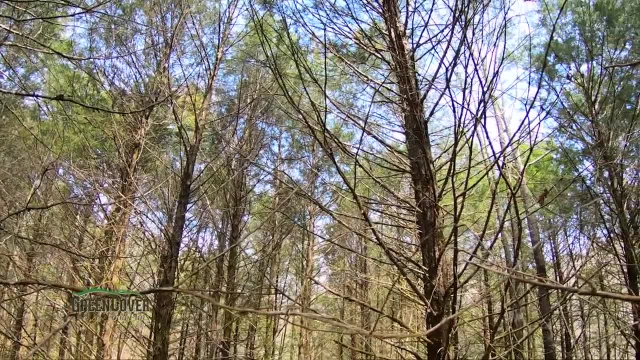 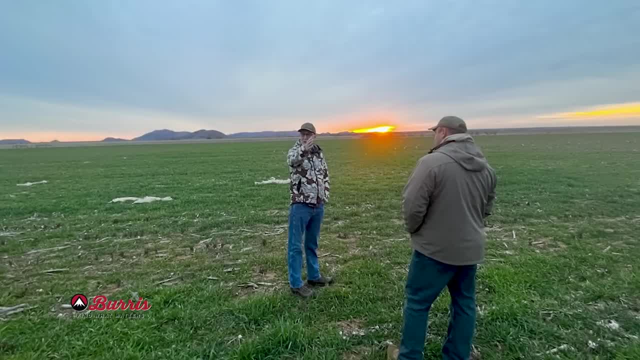 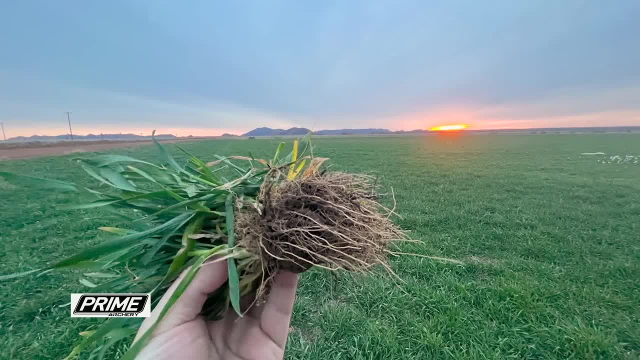 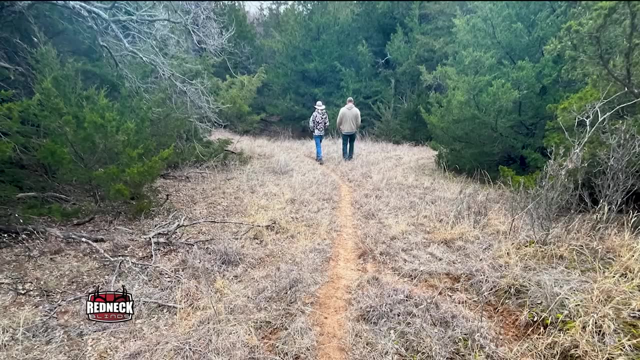 don't know this, but there's a lot of either open land or even wheat land out there. So the areas that aren't tillable or used or grazed heavily end up being cedar. So that's the cover. Deer go there for cover. That's not saying cedar's good cover, It's like you know. I don't necessarily. 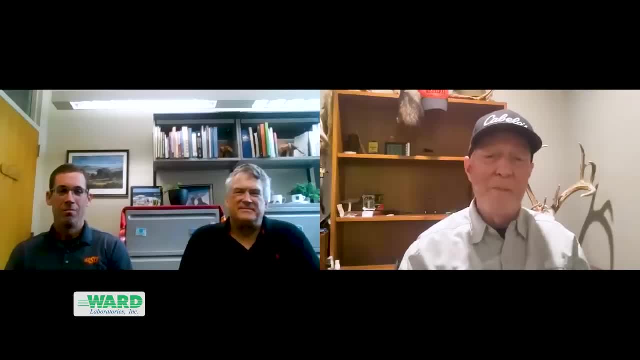 want to eat snail for dinner, but if I haven't eaten in three or four days, snail might sound pretty good. So deer are using these cedar patches out there because that's the best cover around. We're not saying that cedar's good cover, It's just the best cover in that habitat. 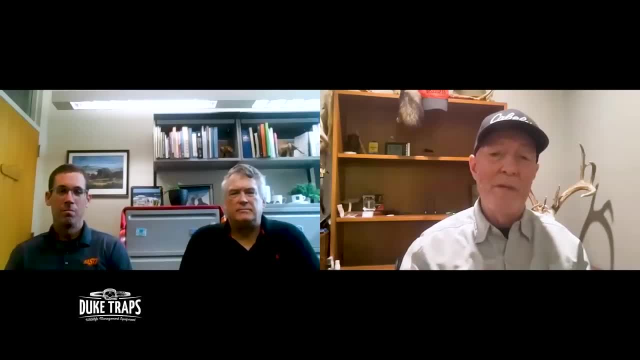 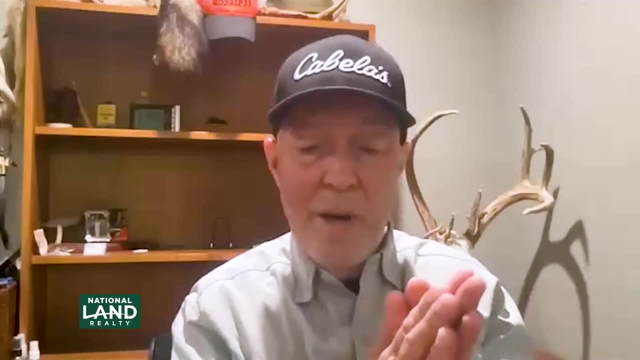 And then deer go in that shaded, humid environment and ticks shed off the deer And voila, we got an active tick population. So you're seeing this, do I understand correctly? You're seeing this trend of tick populations increasing in density in geographic? 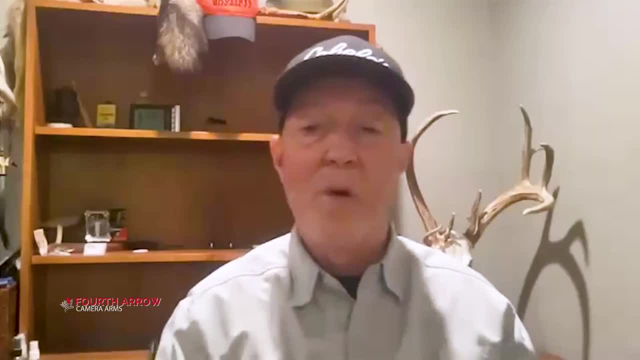 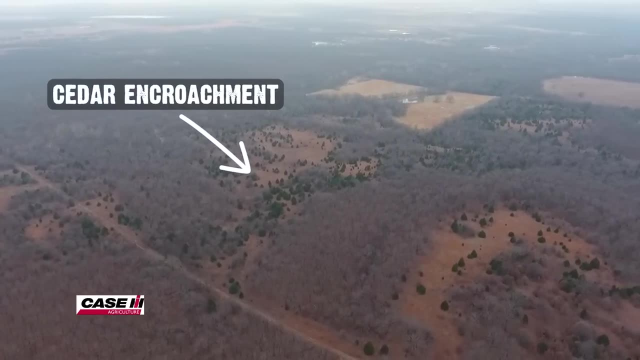 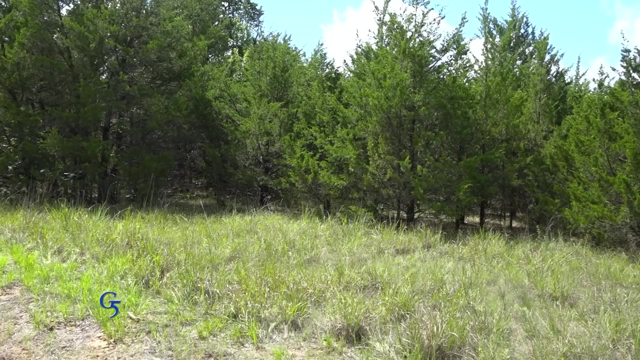 spread going from east to west across Oklahoma. Is that correct? We think we are. I mean, we definitely know here in central Oklahoma where we have the, you know the cross timbers, where we have the post oaks, but we also have the eastern red cedar. 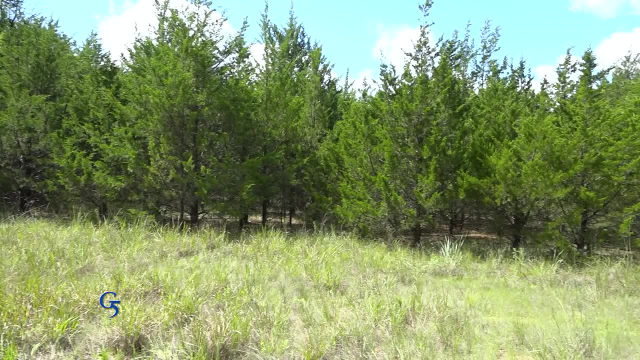 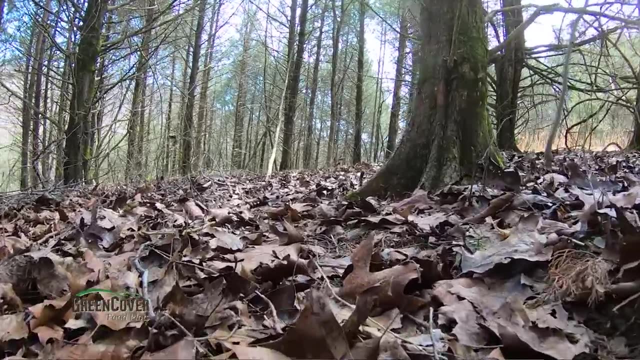 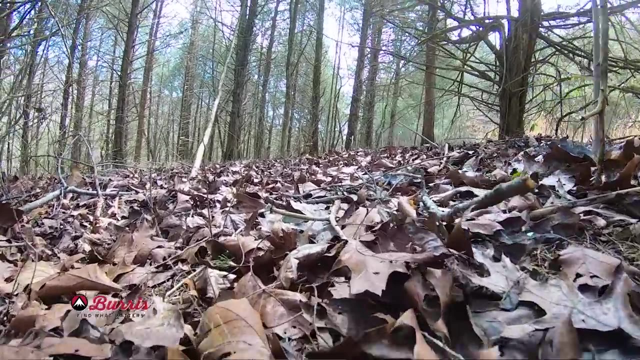 You know, our populations of ticks are quite a bit more in our red cedar areas, but we're hoping. part of the project that we're on now is to see whether, you know, we see this gradient effect And we feel like we are in some ways seeing fewer and fewer ticks as 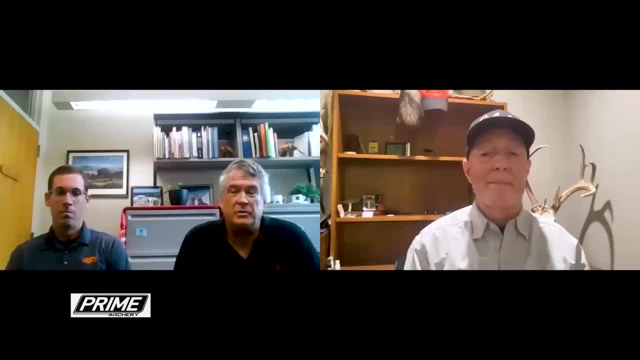 you move west, but we're still getting ticks all the way out to you know, Woodward, Wow, Yeah, I know Woodward. Yeah, yeah, That's discouraging in some ways. Yeah, Would you have any idea that you know if you're a landowner in those areas and you? 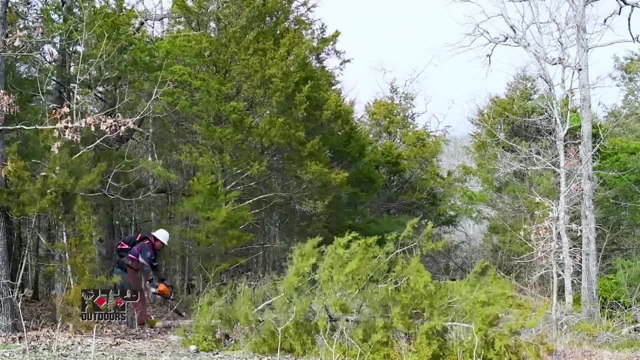 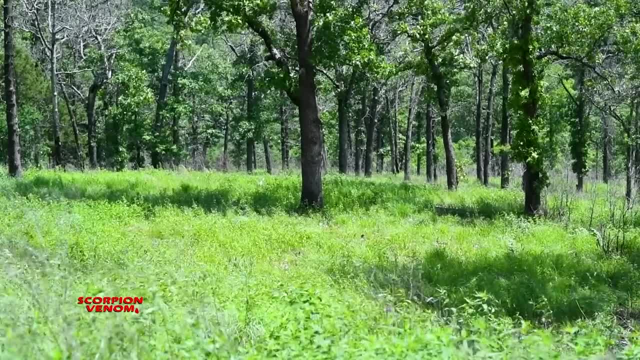 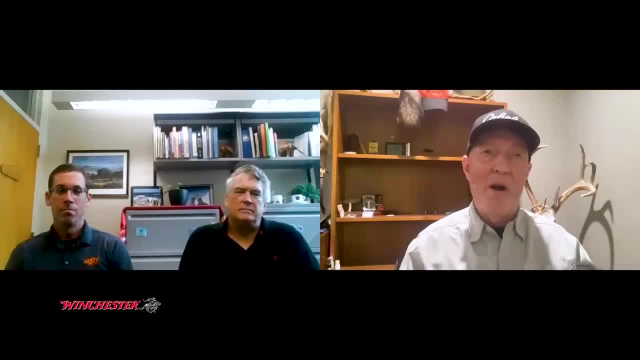 that savanna habitat, maybe in the post oaks area, but your neighbors are not. Are deer going to keep dropping enough ticks in there? Or when you create that environment with less humidity, less moisture will there be? do you think, hypothetically speaking, there could be fewer ticks on that? 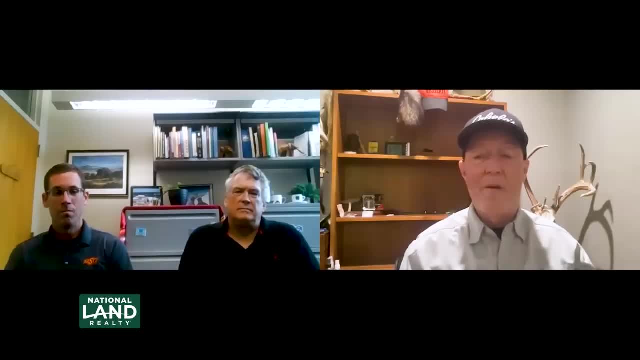 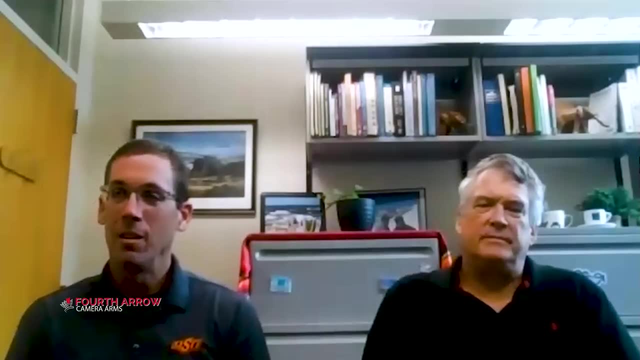 property than there could be on a neighbor, properties that are, you know, crowded out with cedar trees. Can you make a difference on a smaller property? Yeah, so that's really. we do have evidence, especially from Dr Nodin's past work. you know that, compared to being under an eastern red cedar tree, 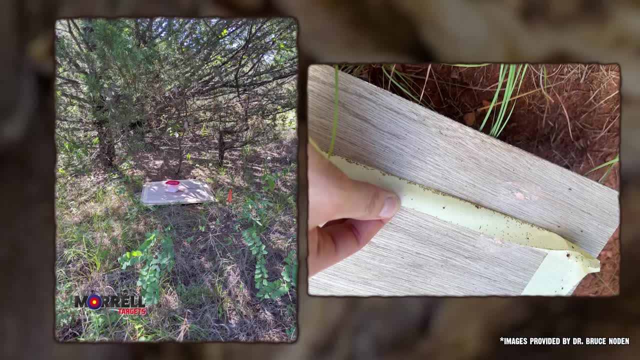 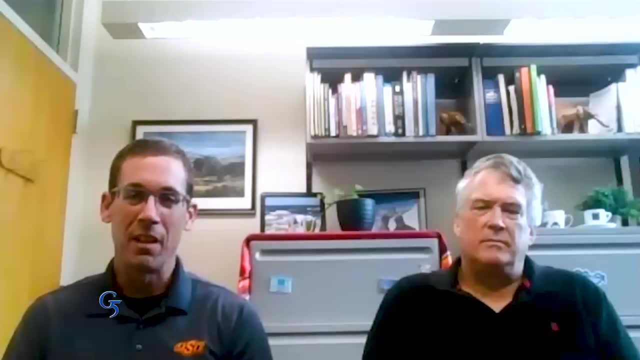 versus an open grassland next to it that you're more likely to find ticks like especially lone star ticks under those cedar trees, But on like the sort of broader landscape. I think that's one of the directions where our research is going. We've scaled up a little bit and sampled at. 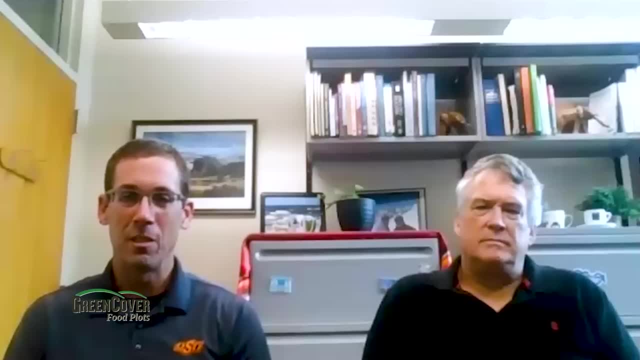 broader sites that have different stages of eastern red cedar encroachment as well as open grasslands, in hopes of comparing, like a sort of broader landscape with different stages of encroachment, what that will mean for ticks across that broader area. We don't have you know. 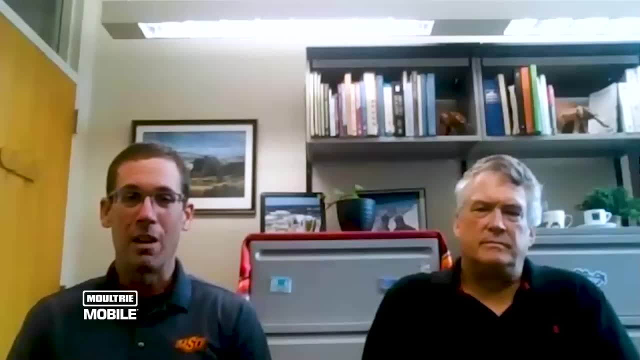 final answers yet, And I think that would be a really crucial question to address, like how much of an area would need to have eastern red cedar control and restoration to these grassland, shrubland and or savanna conditions to like cut them off sort of. on an even broader say, like a county level right, But it's certainly removing eastern red cedar or reducing its cover should at least have local scale effects, we think, On the property where it's done that might not prevent ticks from being on the neighbor's land right And there may occasionally be ticks dropped off from the cedar areas nearby. by moving animals like birds, small mammals, deer, etc. But any amount of restoration would contribute to making a difference, I would think. from a tick-borne disease perspective, That's great information And I think maybe another way to look at that is. 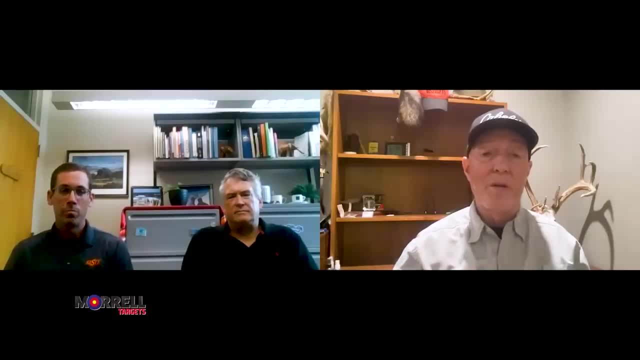 ticks, from my understanding, desiccate pretty quickly. So I'm sure you guys know a little bit about that. Share with us. you know, if we took a vial of ticks, heaven forbid and you know, poured it out there in a hostile environment for ticks, that open grassland savanna habitat. does that significantly reduce your life expectancy because you're in that desiccated habitat? I don't think there's been a study where we've just dumped ticks out there. I think we've done the converse, where we've actually taken ticks and put them into a huge 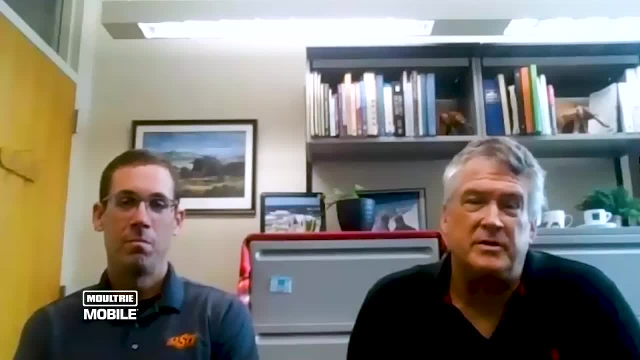 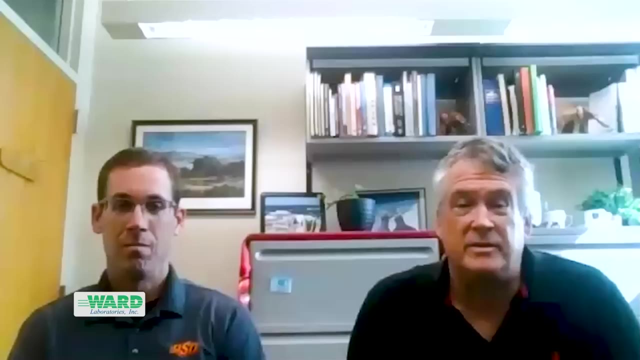 humid area And I don't know if you know, but the Cooks and Hills area near Tahlequah my predecessor took basically recently fed ticks, nymphal ticks- and he put them out there and put them in cages- just environmental cages- and left them And he ran out of funding after. three years. so he had to stop the study. But at the end of three years 29% of the ticks were still alive. So that tells you that the High humidity of eastern Oklahoma is enough to keep ticks alive for over a thousand days. 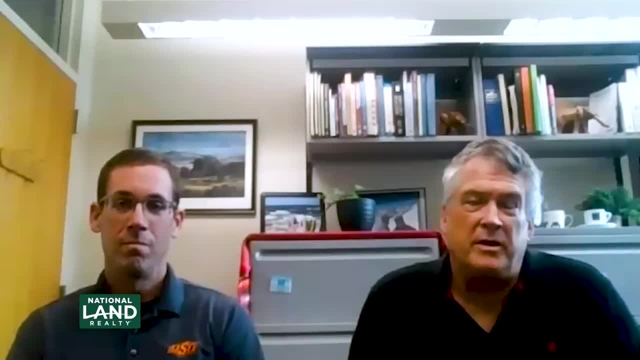 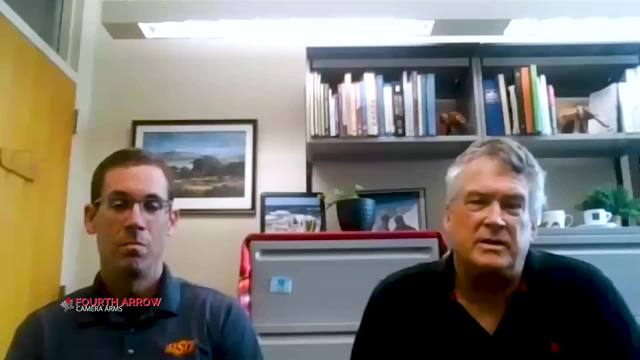 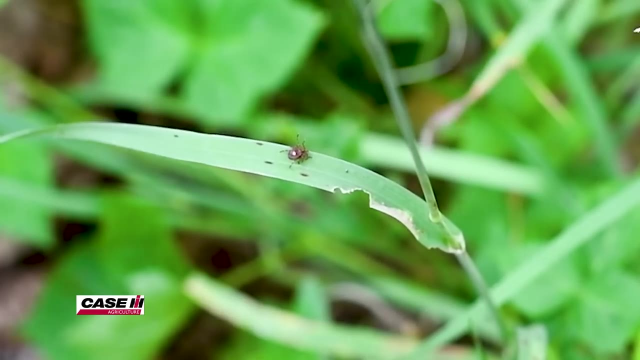 Conversely, we know that one of the things that really moderates tick activity is their loss of body water, And so, essentially, they go out in the morning. you know, you usually encounter a tick about eight o'clock in the morning, nine o'clock. They'll get out there, they'll quest. 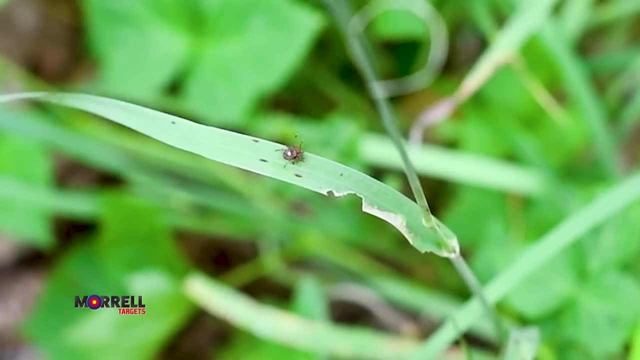 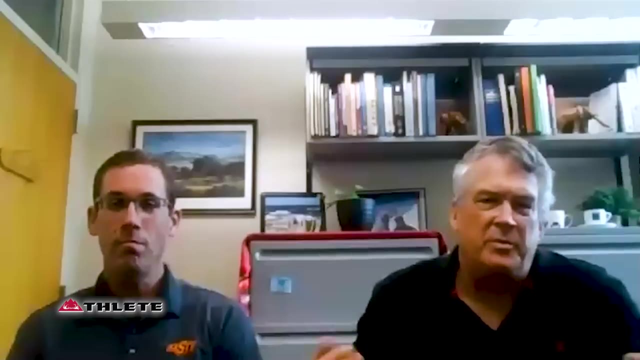 for a while on the edge of the grass. they'll dry out, They'll get out there. they'll get out there, and then they have to go back down into the leaf litter and then they can pick up water from the environment. And so they go down there, they pick it up and they may come out in the evening. 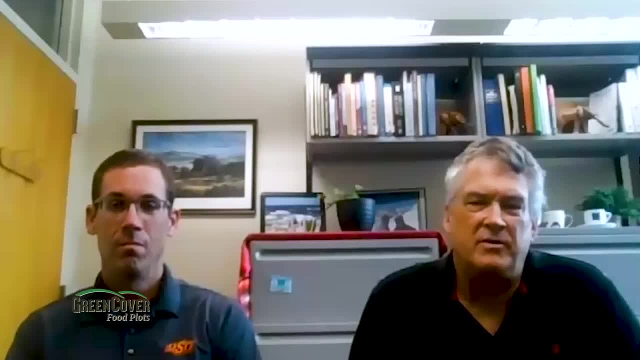 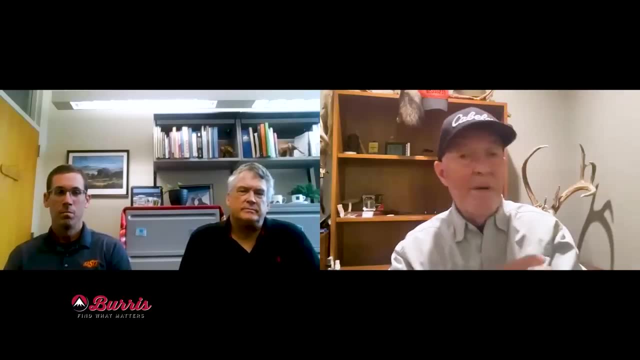 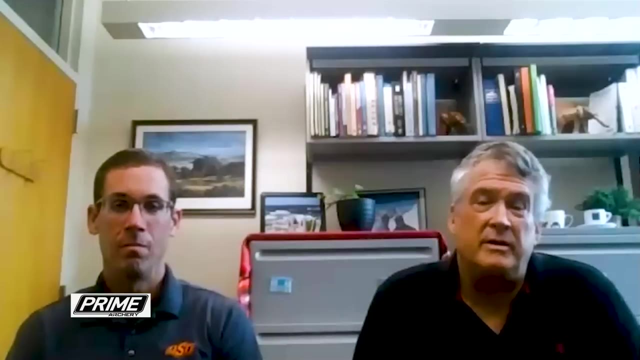 or they may take a couple days, But yeah, they're heavily, heavily, influenced by humidity, And when we're talking water needs, is that keeping their exoskeleton moist or is this? they're ingesting this water. It's actually a percentage of water in their body. If they get below 70% water load then they're at risk of dying. So they get out there. they quest for a while. they sense: oh you know, I'm drying out here, I need to. That's actually one of the reasons why we run into sea ticks in groups, not individually. 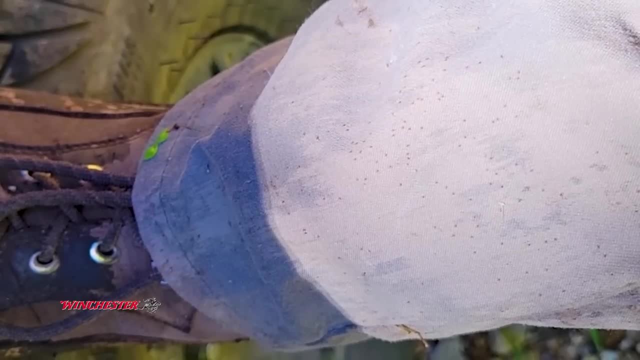 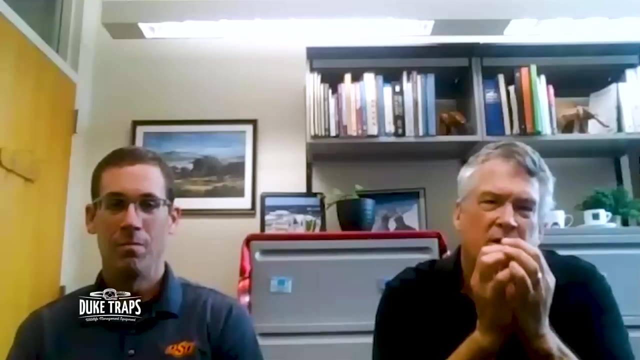 Okay, You hardly ever get one sea tick. You usually get a you know a big bomb of them on your leg or something, And that's because they quest in groups. They actually They quest in a clump, And by being in a clump on the edge of grass they actually keep their. humidity higher and they can be out there longer looking for, you know, waiting for a host rather than being, Because individual tick larvae are very, very sensitive to humidity. Yeah, we notice that we do get those bombs of seed ticks We actually take keep duct tape in. 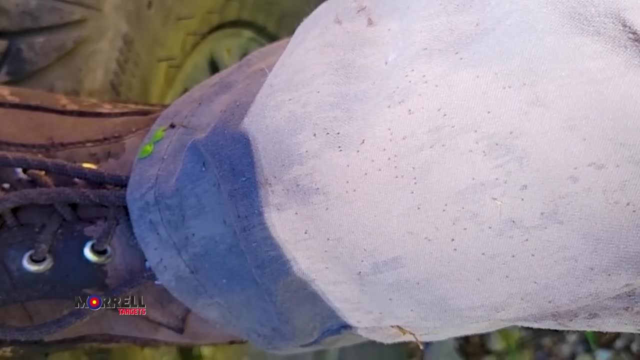 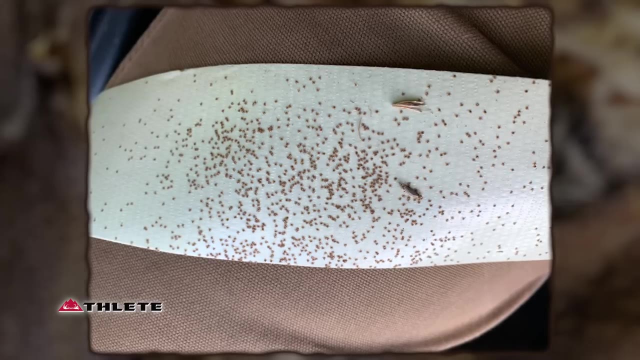 our work vehicles and whatnot, and we're rolling it up right. But if we get a bunch of ticks, we reverse it and just pat ourself Or our pants or whatever, and you'll get. I mean, you'll turn that tape, you know. 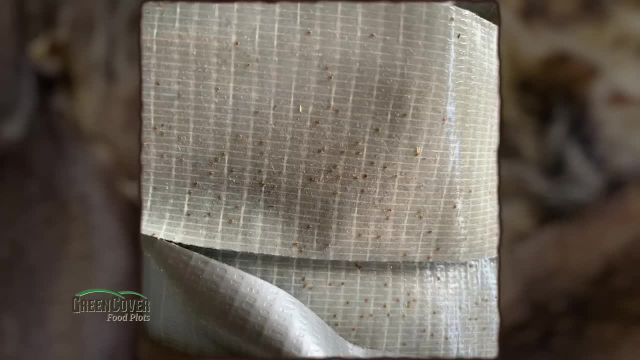 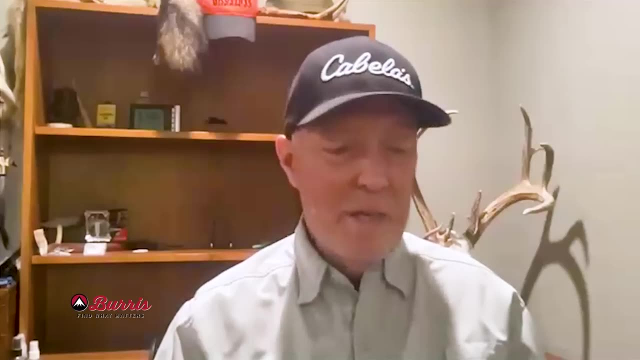 from gray to brown pretty quickly when you get a big load of seed ticks on you. I worked for Squidis South Season Wildlife- the East Cooperative, when I was in grad school And we had a tick study at the Piedmont National Wildlife Refuge and we would put dry ice out. 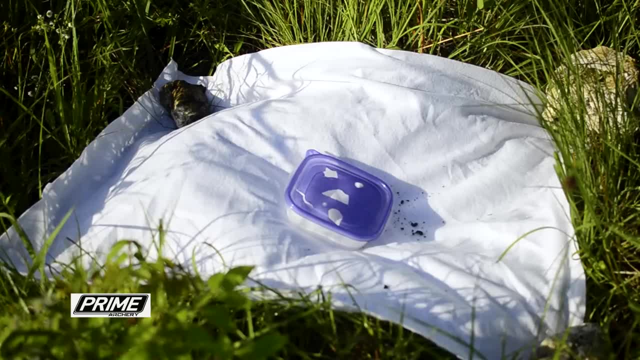 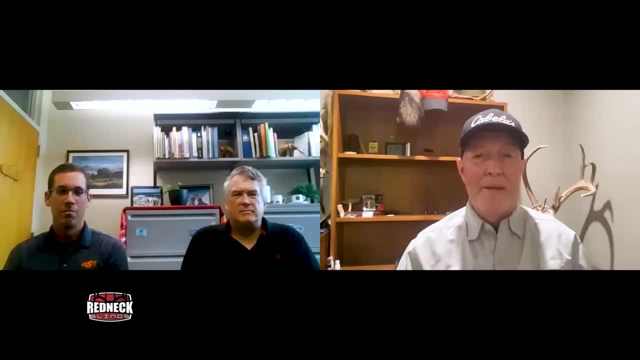 and you know count ticks coming to it for X minutes or whatever, on a meter square of white paper. And I can remember the professor told us to wear white painter pants And I'm like, I'm just going to work, man, I'm going to wear blue jeans, not white painter pants. 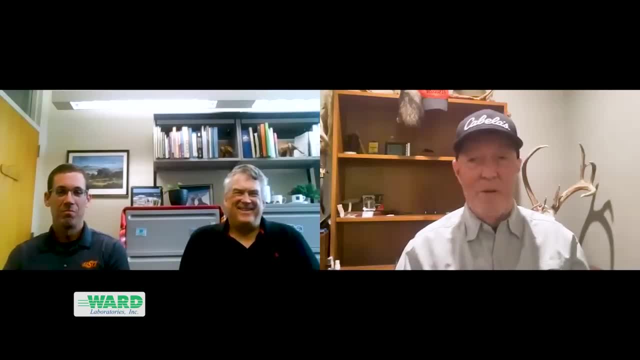 The first day I learned because those students who did follow the professor's hint wore white painter pants and of course they could see the ticks on them instantly. And my blue jeans did not quite show the ticks as much, but we almost collected as many ticks off of us standing. 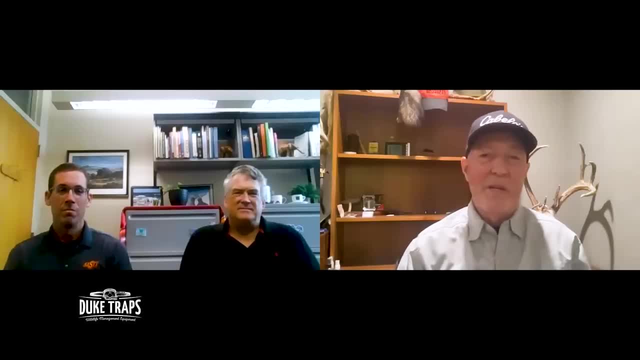 there waiting for them to get on the white plastic sheets so we could count them and catalog them. They were picking us up on the way to that dry ice. So, by the way, as you can all can explain why dry ice attracts ticks to our audience out there. why does dry ice serve as an attractant for ticks? Dry ice is essentially gives us carbon dioxide, and carbon dioxide is exactly what we exhale. So it's basically like you sleeping in a bush and just breathing, or a deer, you know breathing in. 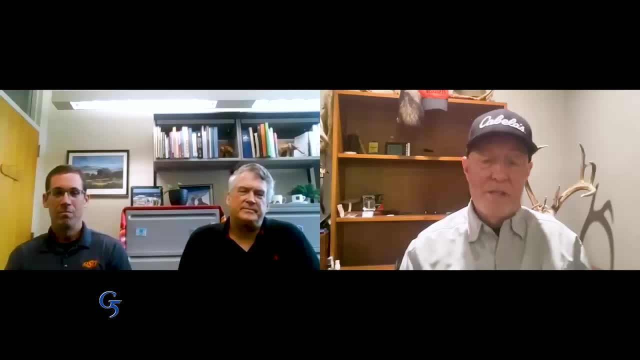 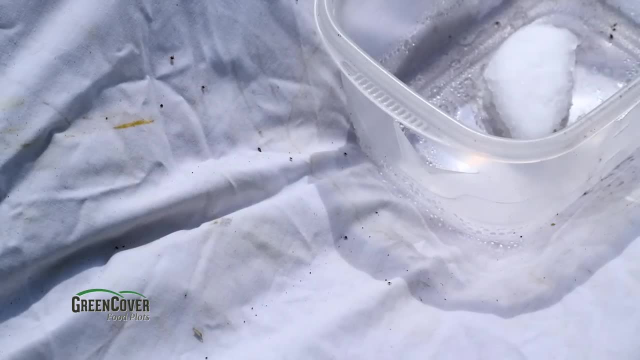 a bush. Dry ice acts the same way. Yeah, So what I want to share we're going to end up after this, but you know, we put just a little chunk of dry ice on a white sheet of plastic and it, as it, melts or breaks down. that's just like. 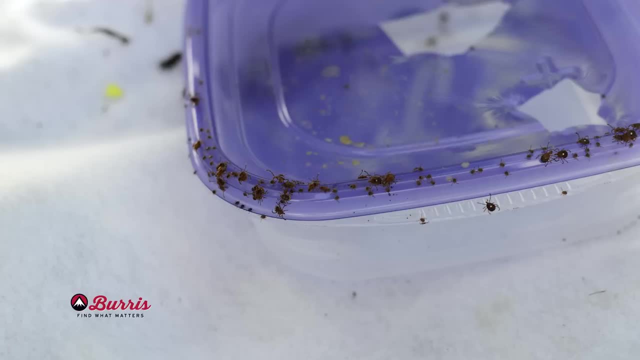 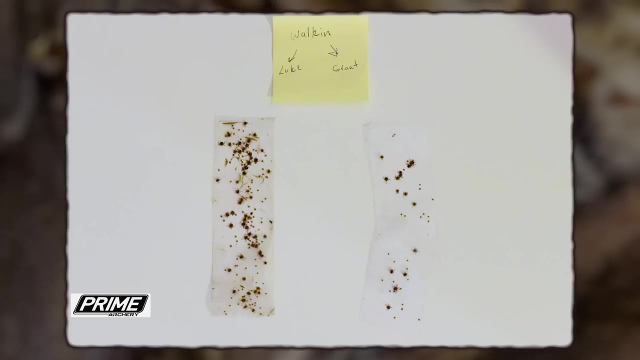 we're respirating or a deer laying there respirating in the white plastic so we can see them easily And we collect them on masking tape. It's not as sticky as duct tape or something. Take it back to the lab. use a dissecting microscope to you know, count gender. 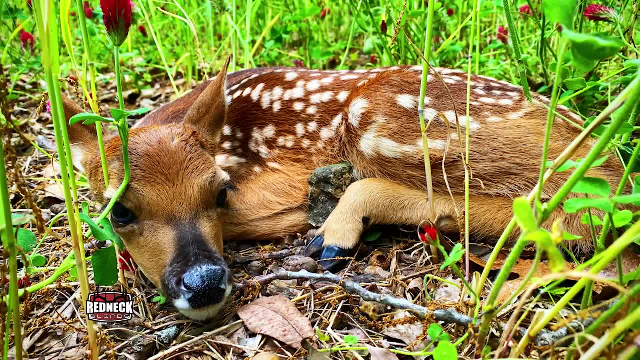 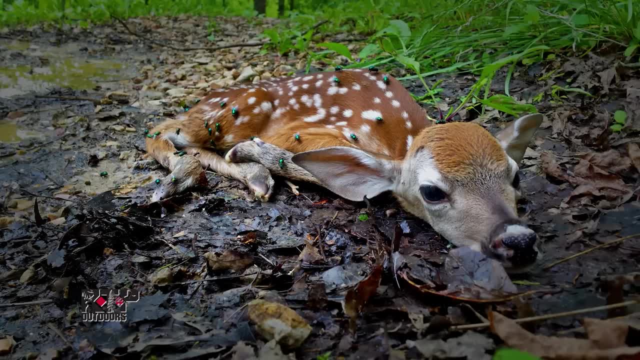 all that stuff for that research project. But you think about a, you know, a four to six pound fawn that's pretty immobile for the first couple of weeks of his life. Well, that's like that, you're that dry ice block just continually exhaling And in bad tick areas. I think it's underrepresented. 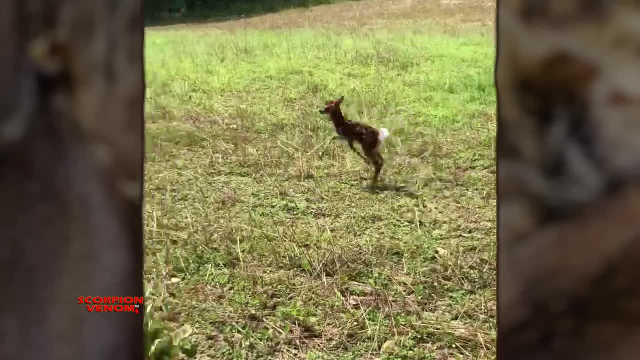 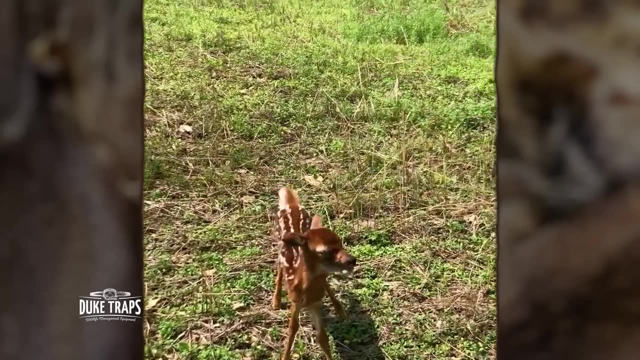 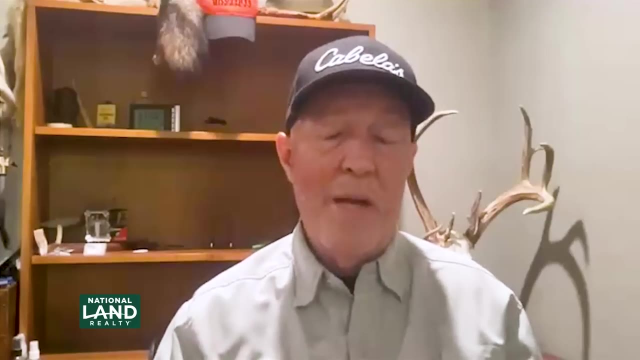 the amount of fawns that are killed by ticks coming to those fawns And they're pretty much immobile for the first couple of weeks of their life. So this is another reason to do good habitat work and reduce the tick populations. if you're into white-tailed deer, because everyone's 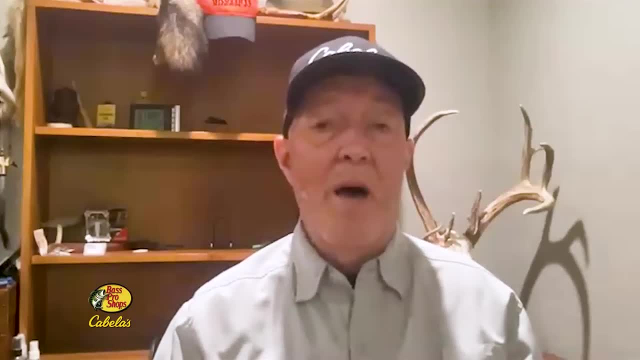 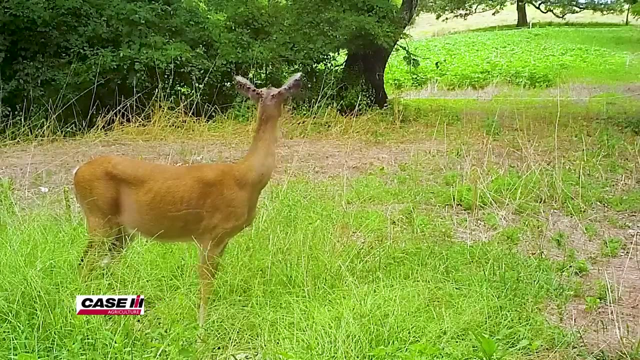 and I do too, but talking about coyotes or other predators, but oftentimes by mass, by weight, the most populous predator out there may be ticks by weight per acre And if you think about, you know a couple of coyotes in a coon. 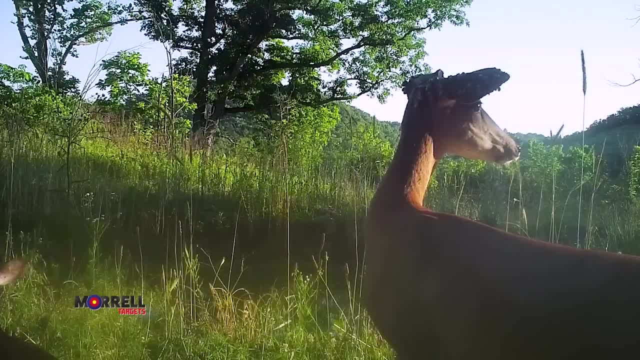 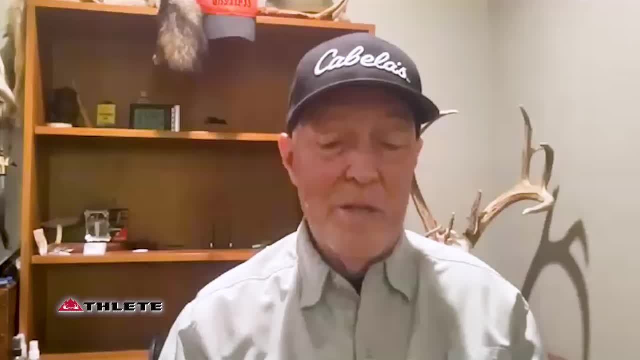 you know, whatever that weighs together- 40,, 56 pounds, whatever it is, you know there could be way more pounds of ticks out there per acre, And so it's. I think tick the research y'all doing is invaluable to the people that enjoy the outdoors. I've had a 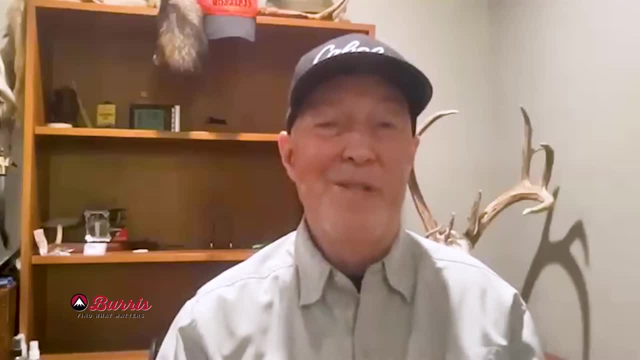 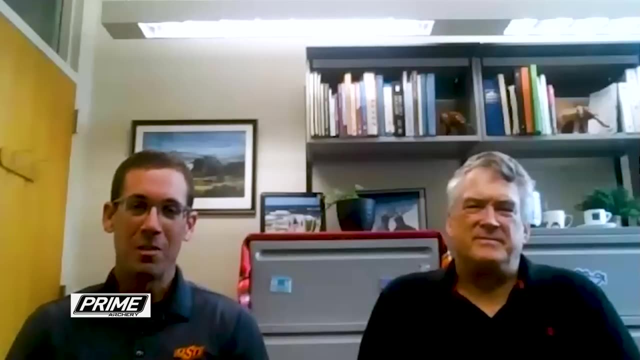 personally had Rocky Mountain spotted fever and rickleiosis, So I'm very sensitive to ticks and I don't mind wearing light-colored pants when I'm out in the field these days. Yeah, Yeah, And so Dr Nodens and my collaboration actually started, sort of randomly. 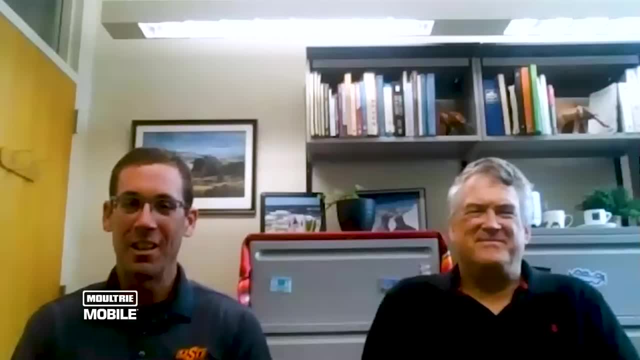 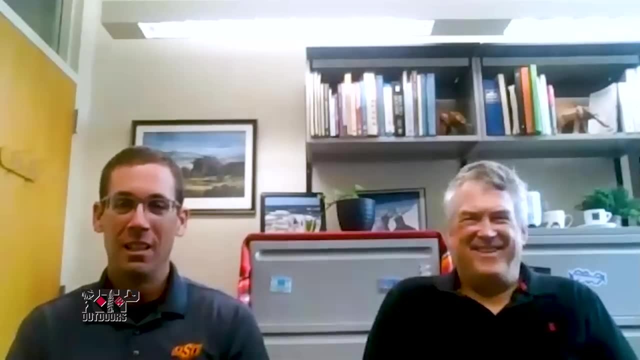 We were both new faculty members here at OSU and we happened to be at a function together and he told me what he studied. I had a little bit of research interest in it, but not much to date. but I did have the personal interest of having caught Rocky Mountain spotted. 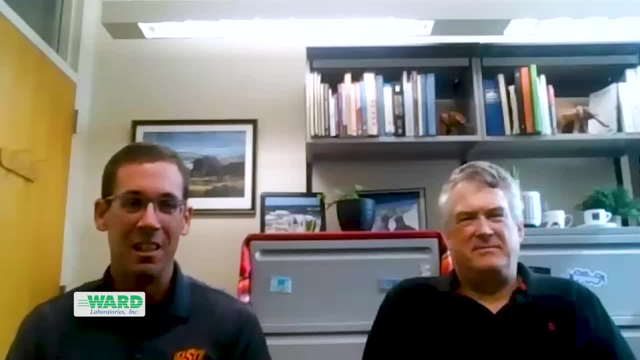 fever my first year living here in Oklahoma, as well as Lyme disease when I had been in the field. I had done field work in Wisconsin previously So and I'm sure there's many viewers, especially from this region from the Southeastern US who are going to have similar stories about having themselves or knowing someone else who's gotten one of these tick-borne illnesses. or increasingly we're getting the alpha-gal bacteria which causes the red meat allergy, which is becoming a bigger and bigger thing. I think maybe there's some confusion about ticks and life cycles I get. 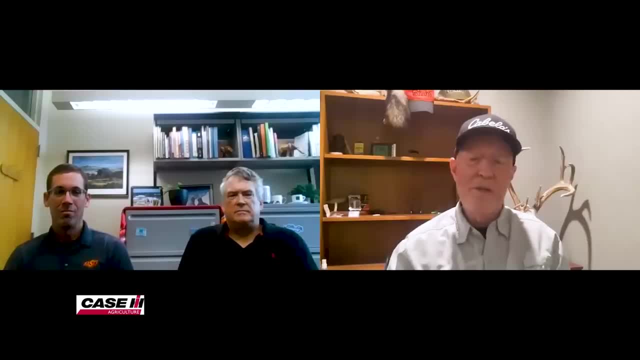 that species of seed tick on my property. So if you don't mind, would you just walk us through the life cycle of common species of ticks we would expect here in Midwest and kind of how they go through that progression? Yeah, I'd be glad to One of the. most of the ticks that we have here in the Midwest are we call three host ticks, And so basically that means that each stage of the development feeds on a different host, And so when a female tick drops off of a deer, she'll usually do it in a habitat. 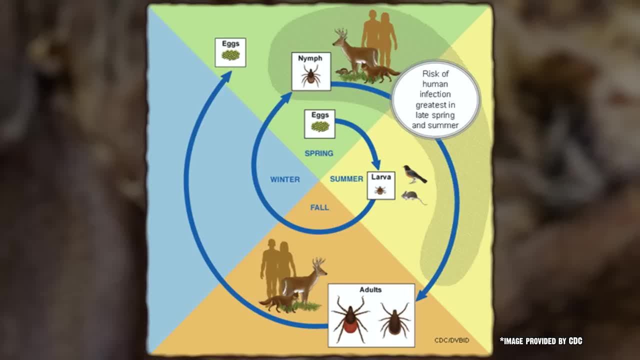 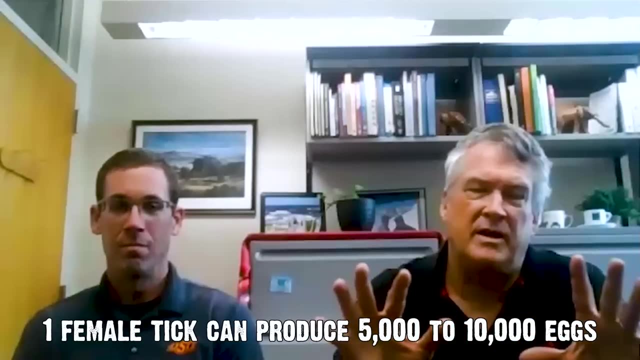 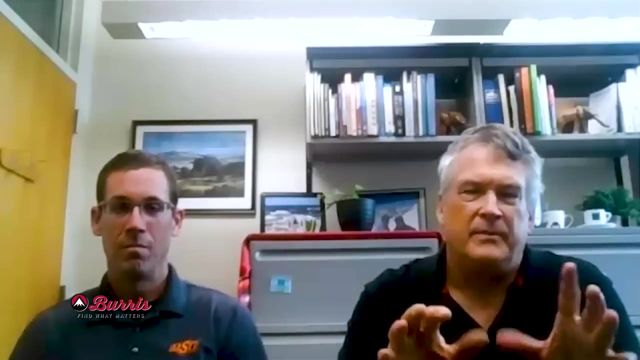 that is conducive to her babies surviving, And she'll drop off the deer and she will put out five to 10,000 eggs And those eggs all get put into one particular area, which is why you get seed ticks all at once, because they all hatch together. And so, basically, when those eggs hatch, 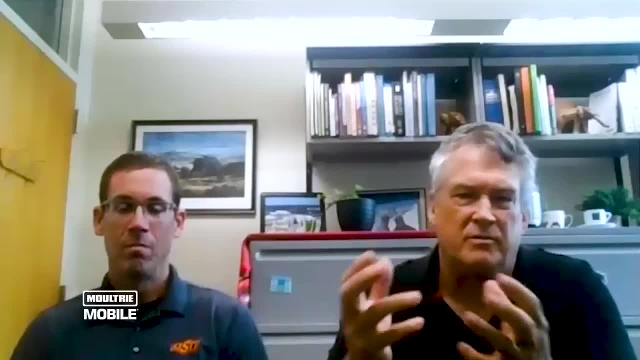 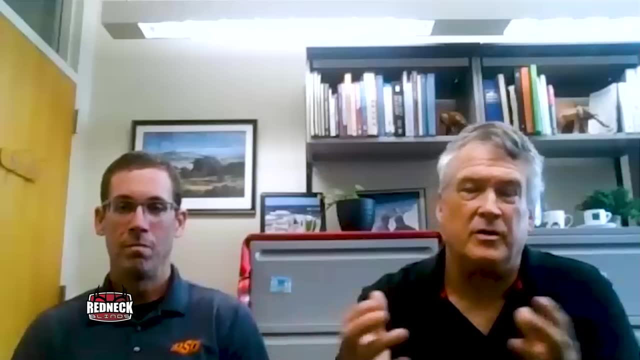 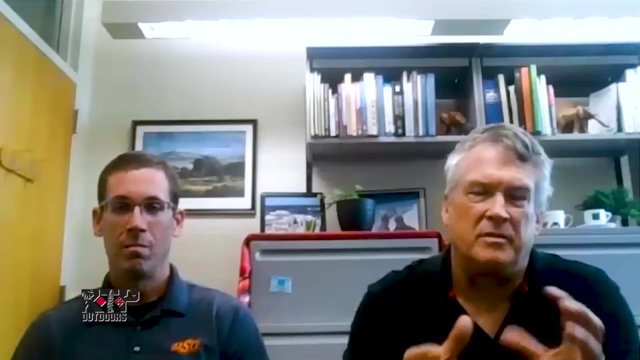 they come out of the eggs and they start looking for a host. A host will come by, depending on the tick. If you're an American dog tick- black legged tick- they'll be on smaller mammals or reptiles. Lone star ticks don't care. They'll get on birds, they'll get on deer, It doesn't. 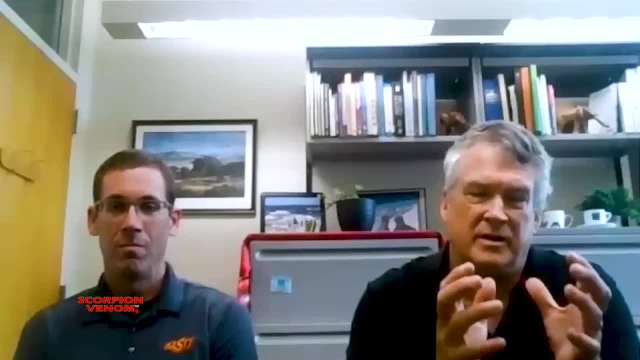 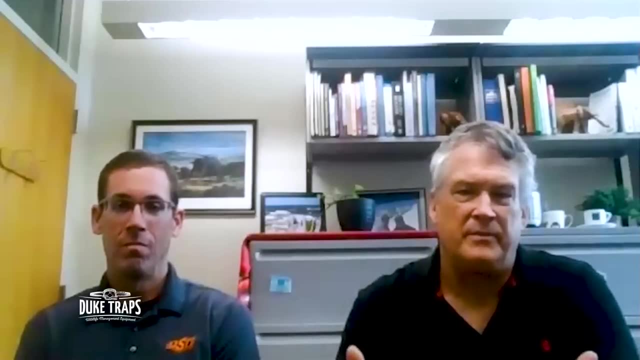 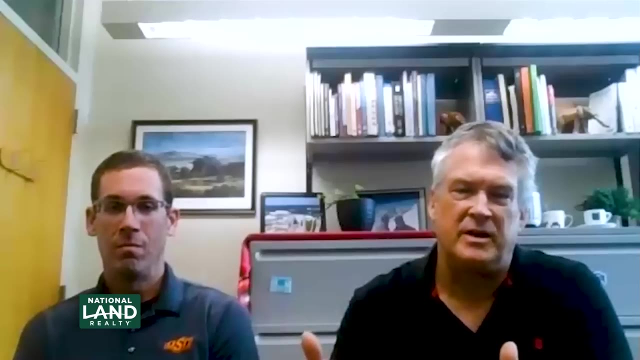 matter what stage. So the seed ticks or these larvae larval ticks get on a host, they feed and they'll drop off into a habitat. Then they will molt and become a nymph And that nymph is not sexually active. It's basically got four legs, It's got eight legs And that stage. 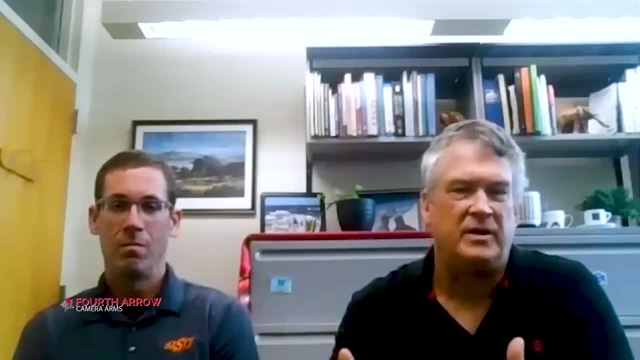 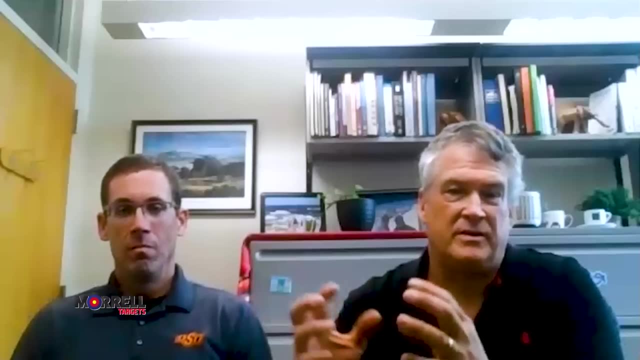 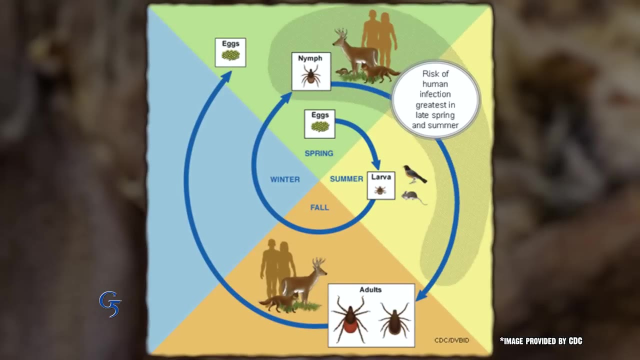 then again, is going to find a host, is going to feed on that host, going to drop off of that host, and then it will molt. And that's when we get the sexual dimorphism, Where we get the males and the females. So you go: seed ticks feed, molt nymphs feed. 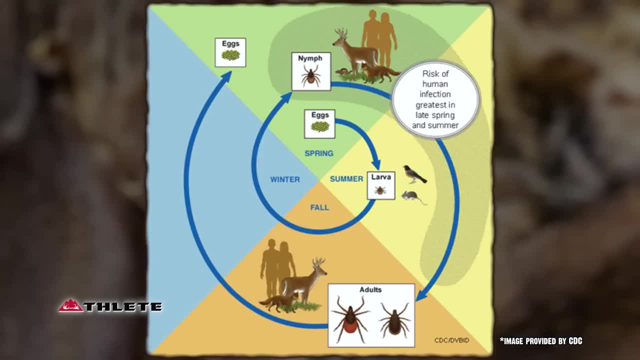 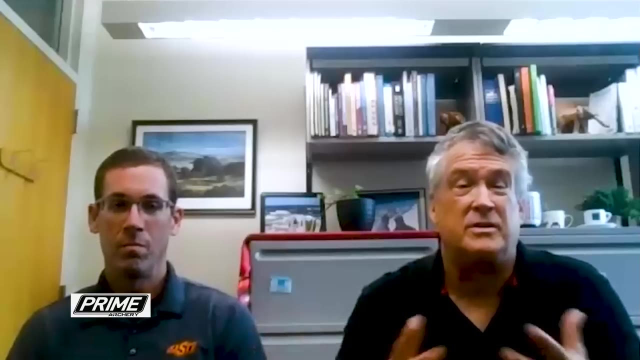 molt adults And then the males and females then will feed and it keeps the life cycle going And that whole cycle will take two years, And so it's really important to, and then, as I said before, some of these ticks are actually going to live for years, So you can have. 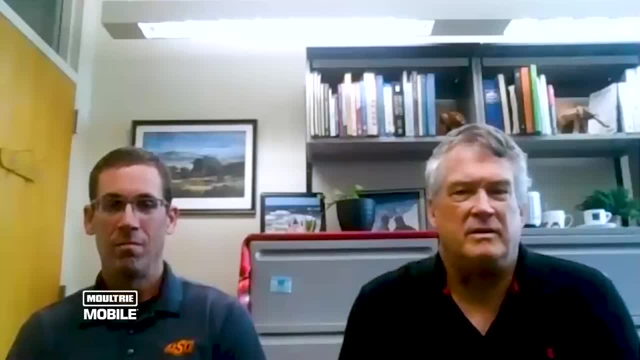 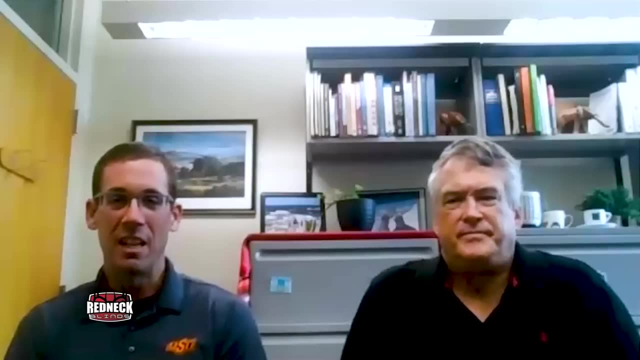 generations and generations of ticks happening in your backyard, And the takeaway related to seed ticks, I guess, is that that's not a species, That's a life stage right, So it could be any number of species that you're encountering in that sort of seed tick. stage? Yeah, What's a common tick predator? What eats ticks? That many of our wild bird species can eat ticks. It may not be a major food source for most birds, but there's a lot of our insectivorous birds that eat gross things like spiders and millipedes etc. And there's evidence. that they'll eat ticks too, including off of themselves. For most of the species of ticks we find on birds they show up right around the head- Not all species, unless many birds carry ticks all over their body- but suggesting that the birds are able to find the ticks and pull and preen them off. 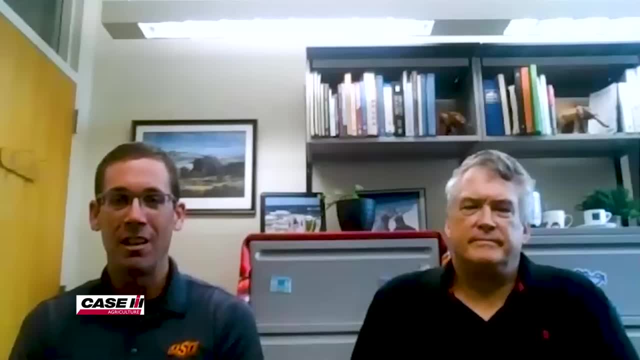 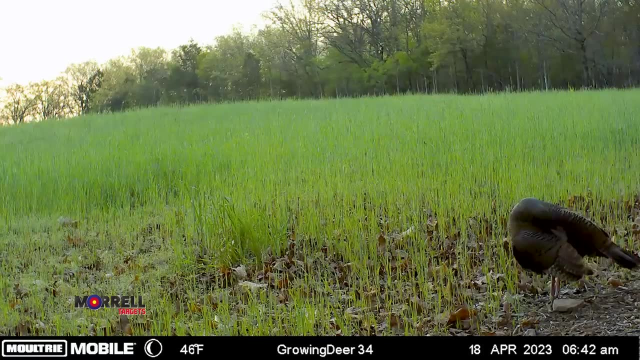 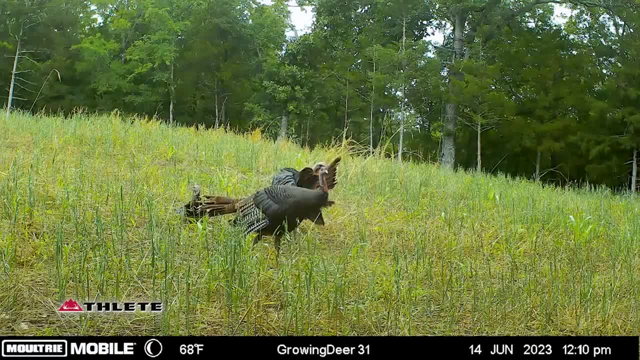 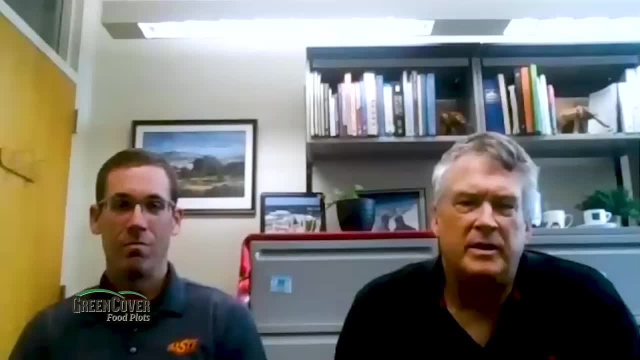 feathers and whatnot. So you've explained the life cycle of ticks. How could you disrupt that life cycle? What's some actions that we could take to potentially disrupt that life cycle? Well, anytime that we can dry them out- We've talked about the fact that they're very 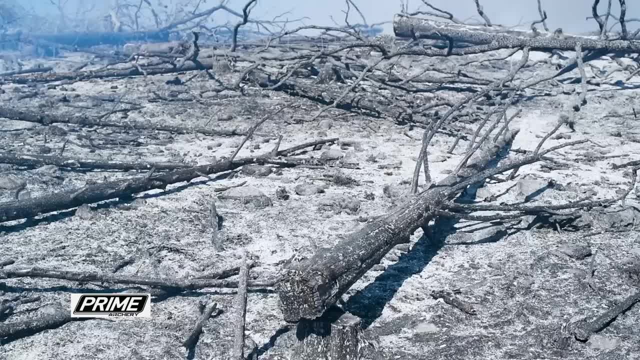 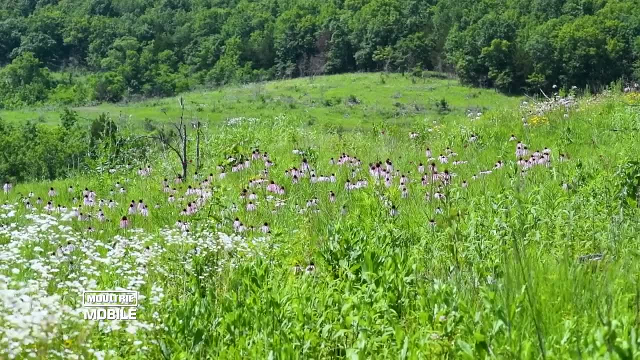 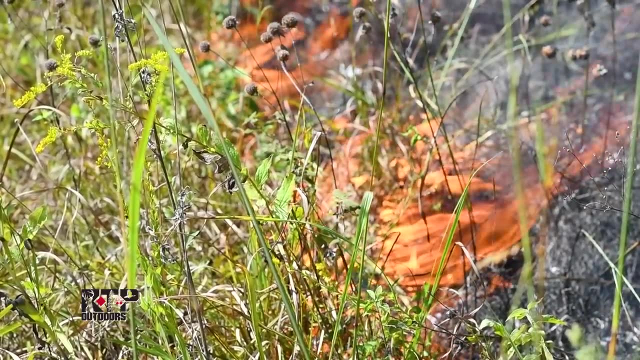 sensitive to drying. So burning, opening up land, that kind of thing, is going to be something that you're going to break the cycle. You have a better chance of doing something to that tick while it's waiting for another host or molting and it'll dry out. So that's why burning is good, Opening up. 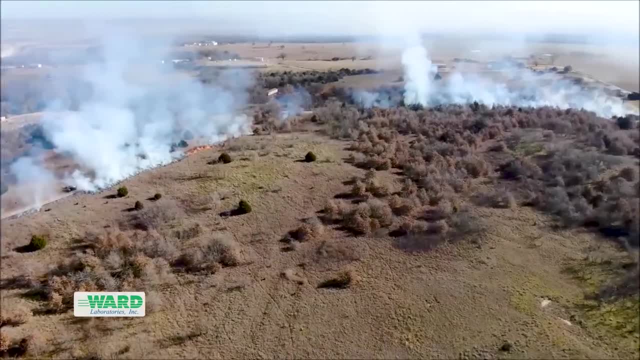 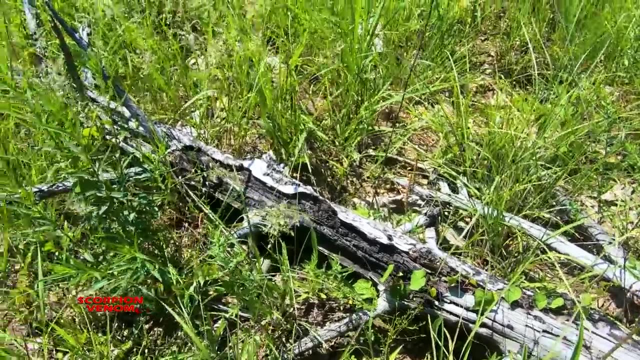 your land, getting the cedar off of it. That's all going to help to create an environment where the ticks are not going to survive as well. I think an intriguing idea that I don't believe it's been researched is that the larval tick or the seed tick season comes near the end of the 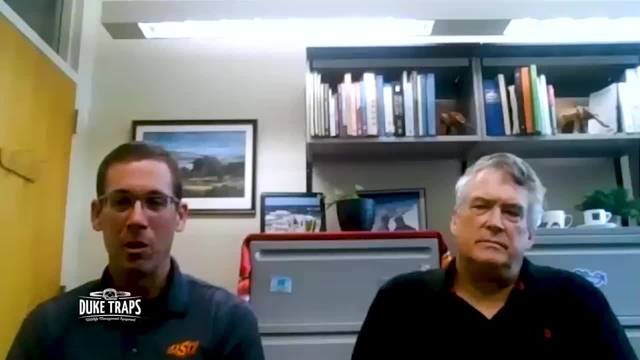 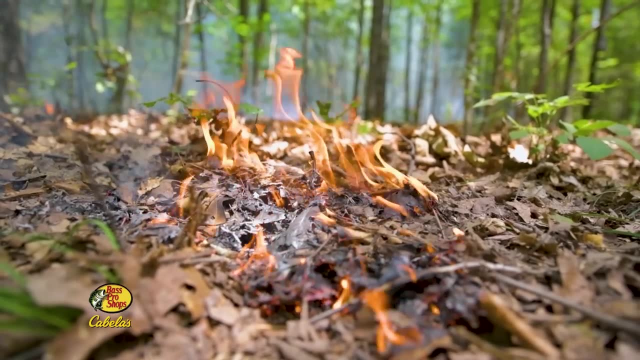 summer right, And there's increasing, you know, increasingly. we know of some benefits of picking about growing season burns. There's evidence that fire, whenever it happens, may actually cause some direct mortality of ticks right. It changes the habitat in ways that disadvantages 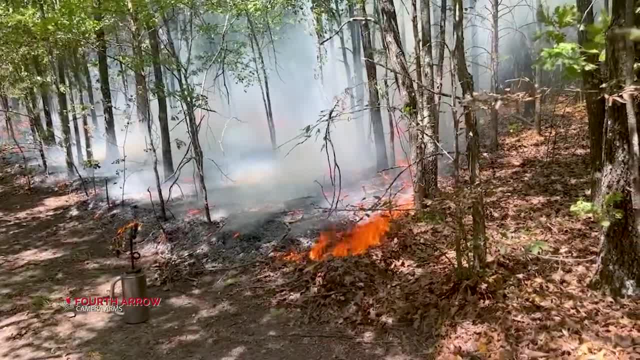 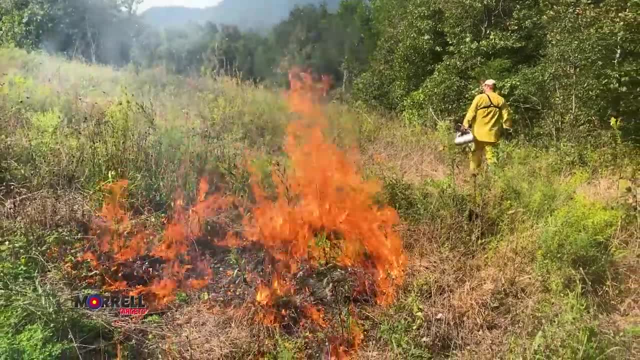 ticks, but some of them also will just be directly killed by the flame. And a neat question to potentially ask is whether the growing season burns might potentially be able to directly kill some of these seed ticks. But as far as I know, we don't necessarily have an answer for that. in our region. You know when I was a boy I heard frequently: oh, we had a late frost this year. Ticks won't be bad. It seems like they were always bad. So can you address whether potentially a late frost might significantly set back tick populations? 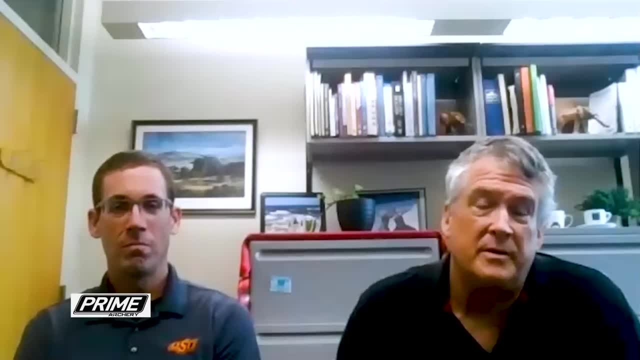 That's a very good question. One of the things that we know is that particularly seed ticks are are. you know, the larval ticks are quite sensitive to temperature. So if you can, if that frost can happen, you know, it normally will knock down the the larval ticks more than 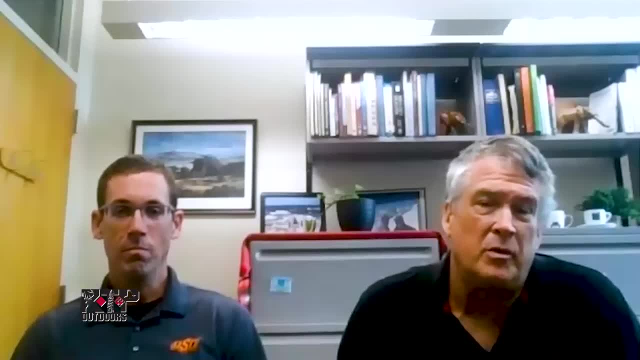 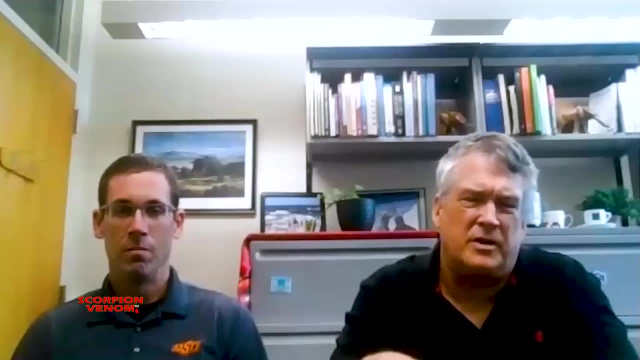 the antler ticks. So it's a very good question And I think that's a very good question. The other ones, the nympho and adult ticks are more- are are able to. you know, they can get into the bases of the roots of the grass or they can get underneath that leaf litter. I mean, I've I've had ticks that are literally dirty. They have dirt all over them because they've been so stuck down in there. And often you know that frost, we think about it because it coats our car, but you know that that frost line has got to get into the soil and into the leaf litter. 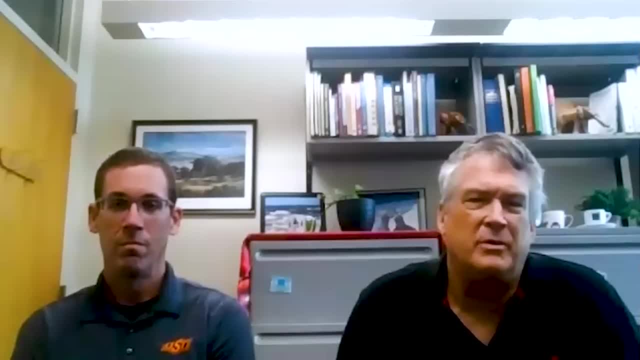 Under those trees in order to make a difference, And that's why we don't see. the difference is because the trees create this environment where the frost isn't going to affect them as bad. So, especially a cedar tree, like we've been talking right, You know, you almost never see. 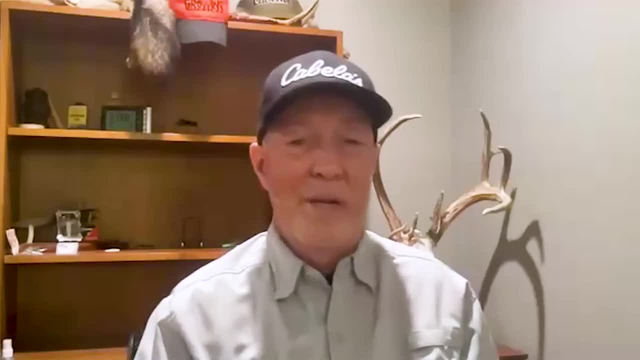 frost under a cedar tree. So that's just another reason to snip those rascals off and put a fire in there, because it's a safe haven for ticks during that situation. Well, Jim and Owen, thank you so much for your time today of sharing with us your work. 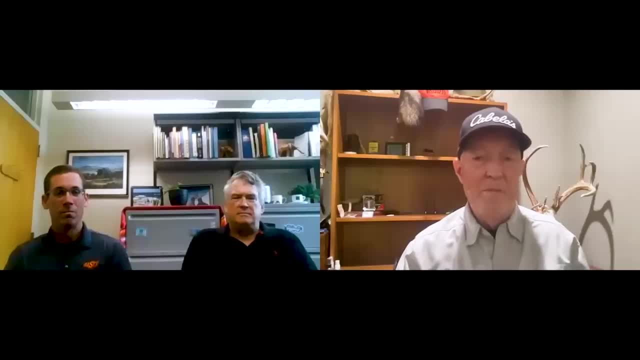 And I would ask you to you know when you're a little bit further down the road, have a little bit more research you could share. maybe come back and share those results with us. put some more checks in the boxes there. We'd look forward to hearing that and helping educate other people. 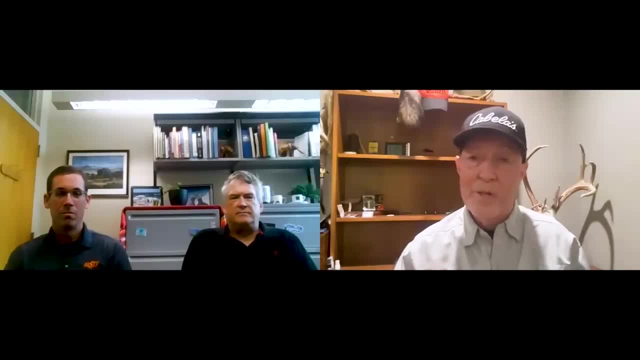 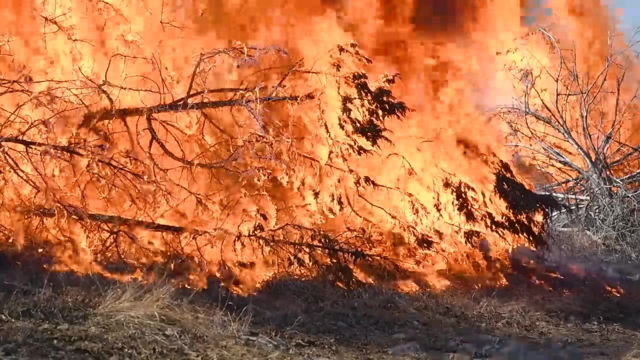 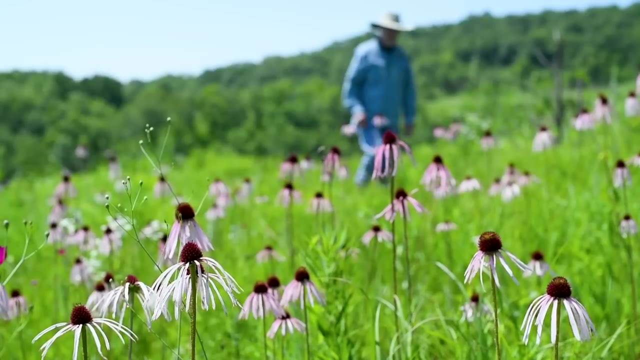 that enjoy the outdoors, of how we can work or encourage our state agencies and federal agencies to manage land And- and I find that when we restore habitat to native habitat- what these early explorers wrote about- there are many benefits to the whole system, And one of those benefits is reduced tick populations. 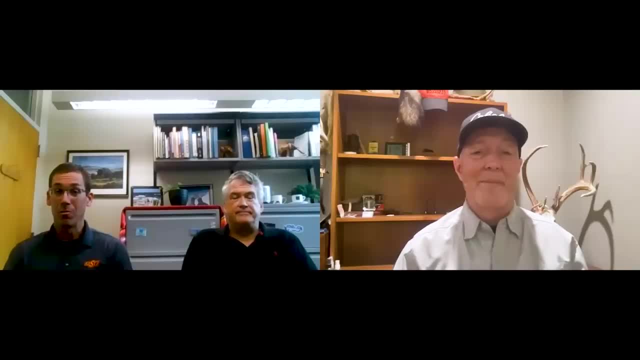 Yeah, You know, there's just lots of mounting research from this region, a lot at our university here and other universities showing that this eastern red cedar encroachment obviously affects livestock production because it takes up grassland, It's affecting potentially water tables and 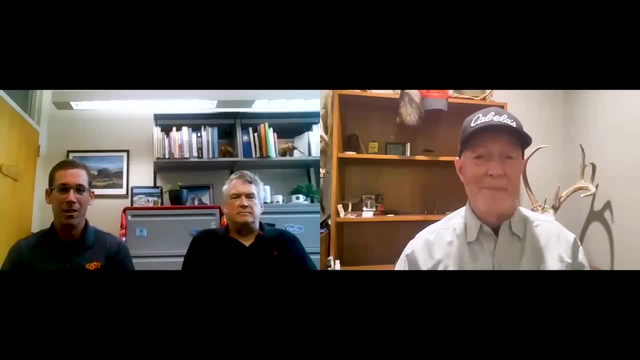 water runoff to streams, because it uses a lot more water then and it intercepts a lot more water. Um it, when it gets to a late stage, it creates. you know, it's, it's, it's, it's, it's, it's. 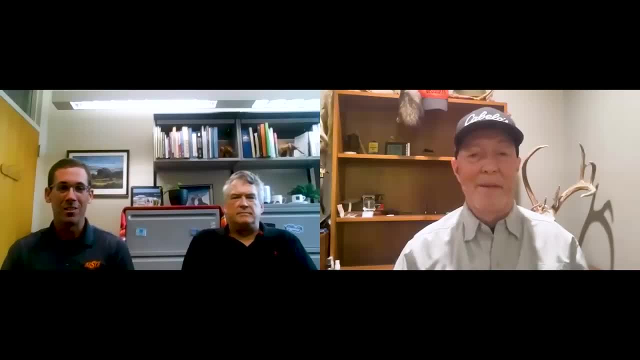 when it gets to a late stage it creates a wildfire risk right. So there's a lot of the disease risk that Dr Nodin has shown over the last few years and that we're looking at is just another sort of important reason to consider restoring the afterway from eastern 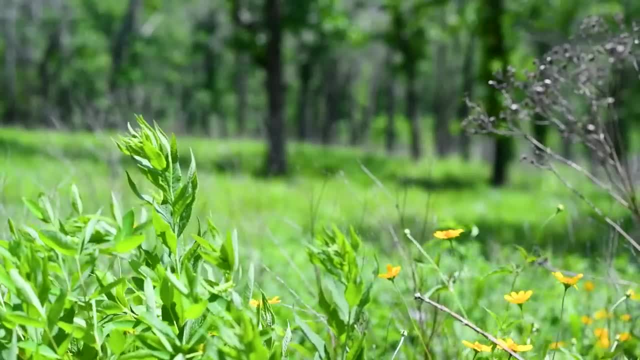 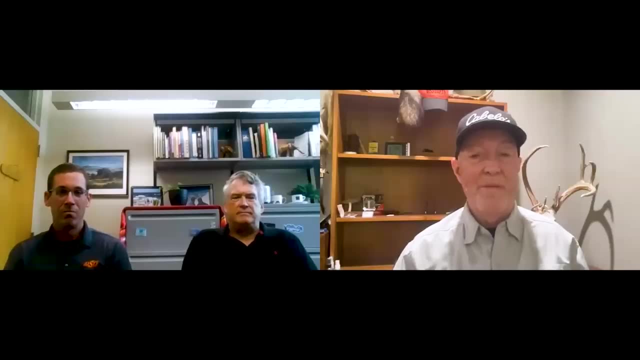 red cedar dominated areas to grasslands in our savannah- native savannahs, I agree. Native savannahs- a very beautiful and productive habitat and probably a little safer for fire tick and a lot of other reasons also. Gentlemen, thank you again. We're looking forward to staying in touch and hearing from.